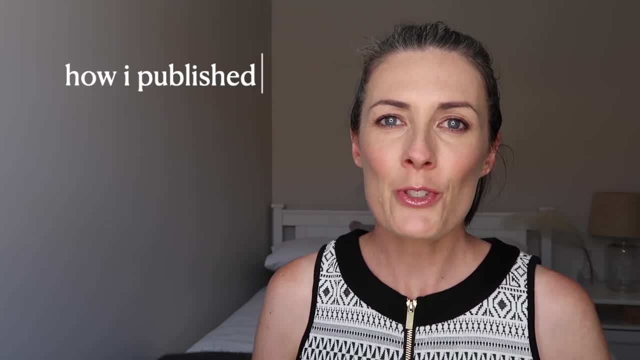 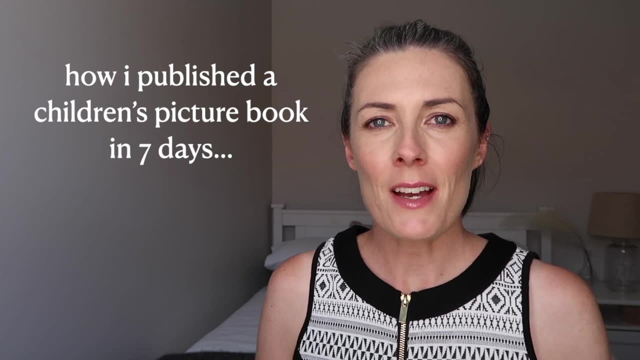 In this video, I want to give you an update on the children's book that I created and published in just seven days, and how I did it. Welcome to my channel. my name is Caroline and I make videos to help you master your mindset and make money online so that you can build a life you love. 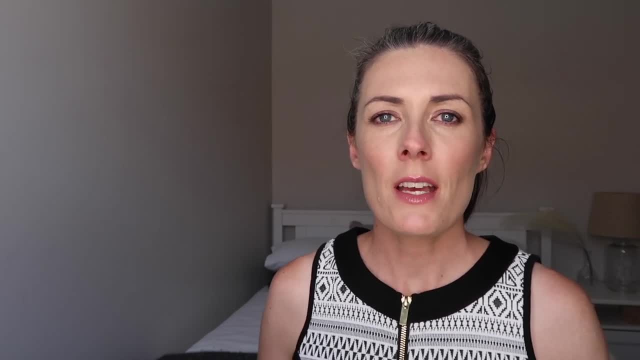 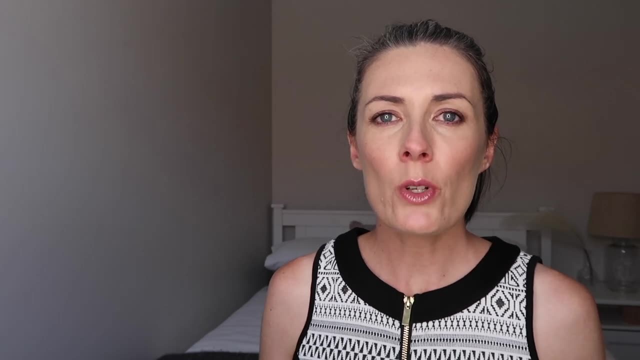 So recently I did make a couple of videos where I was talking about that I was creating and that I was in the process of publishing a children's book and how I was going to do that. I will link to those videos in the description below and at the top of the screen if you haven't seen those. 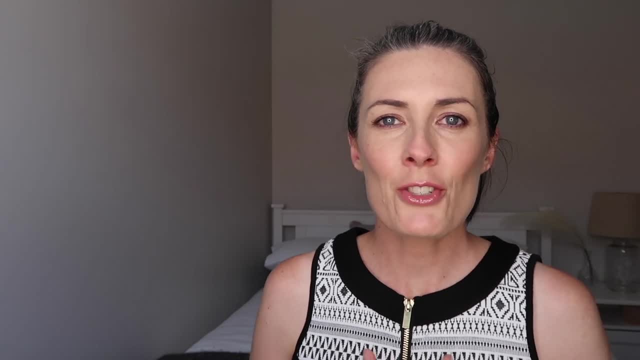 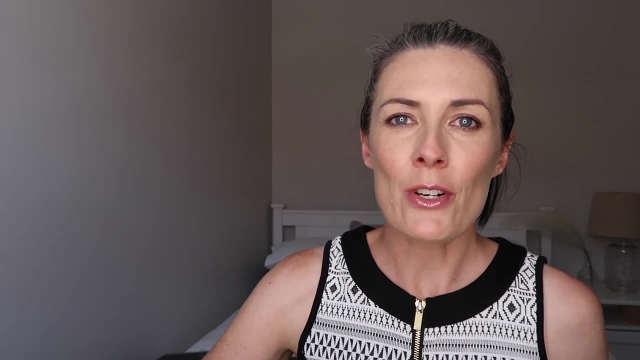 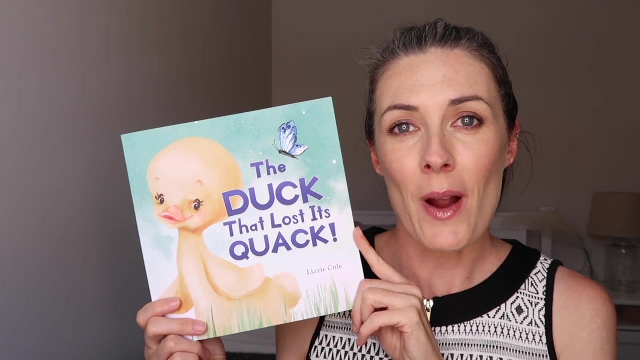 videos and you want to check those ones out. But first let me show you the book that I created, because it is done, it is finished, it is published and it is selling on Amazon. So here is my children's picture book and it is called The Duck That Lost Its Quack. This is a children's 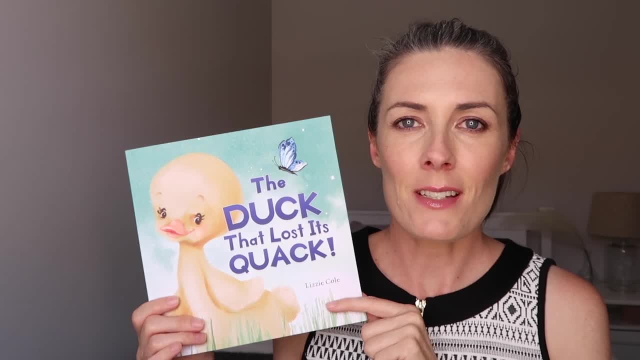 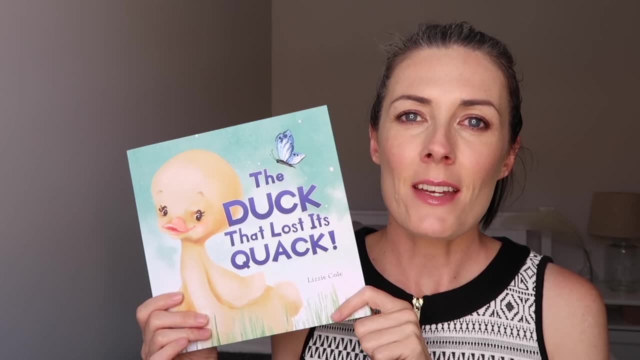 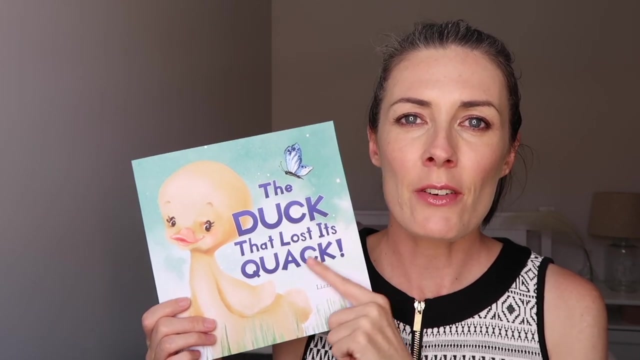 picture book aimed at kids around three to six years of age, and it's a story about a duck who gets a little bit lost. she loses her quack and she enlists the help of some really cute little farm animals to help her find her quack. And so there is a little bit of 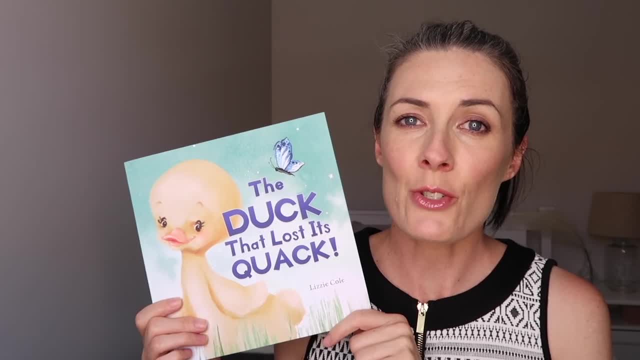 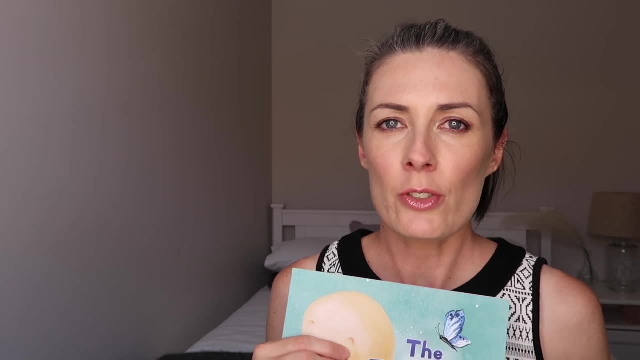 learning about the different kinds of noises animals make within the story. So I wrote this story over a day or two, and then I illustrated the book myself- and no, I am not a professional or even an amateur illustrator. I had never illustrated a book before, while I do have. some skills. So I'm going to show you a little bit of the story. So I'm going to show you a little bit of the story. So I'm going to show you a little bit of the story. So I'm going to show you. 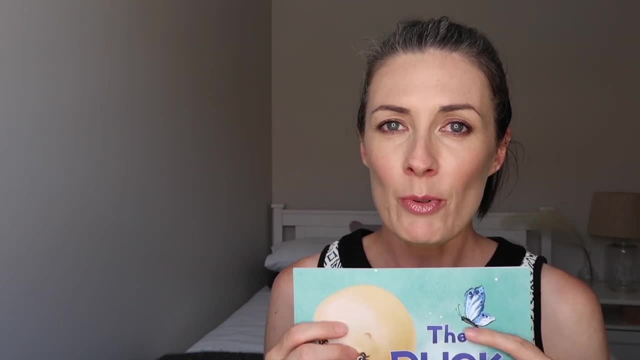 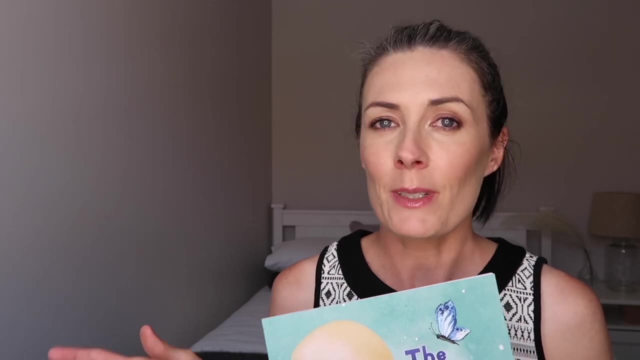 a self-taught background in graphic design, I've never done anything like this before and I didn't pay anyone to help me with any aspects of the book whatsoever. So I will get into that process a little bit later in the video, And I also created the cover myself, But I love how it. 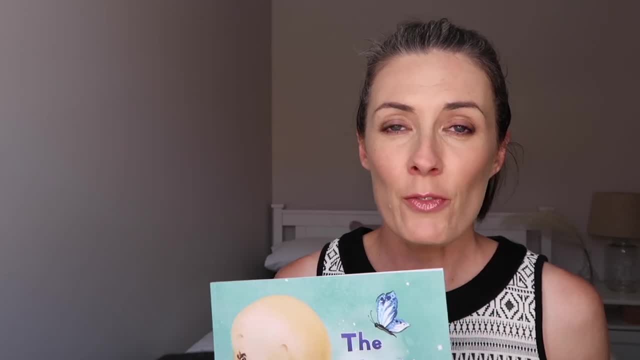 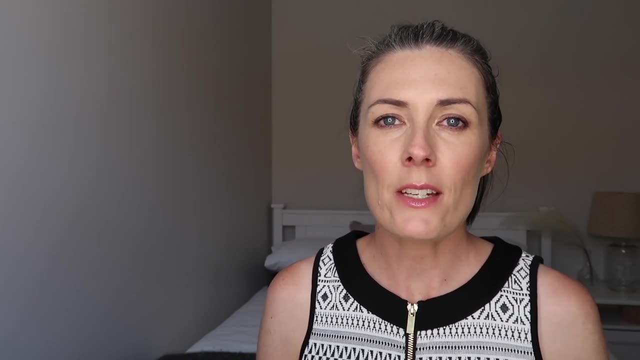 turned out. I am really happy with it, particularly as a first-time published children's book author. So how did I do this? Well, first of all, I did take a course. I took the children's book creator course, which was created and run by my lovely friend Nuria from the Home Boss YouTube channel. 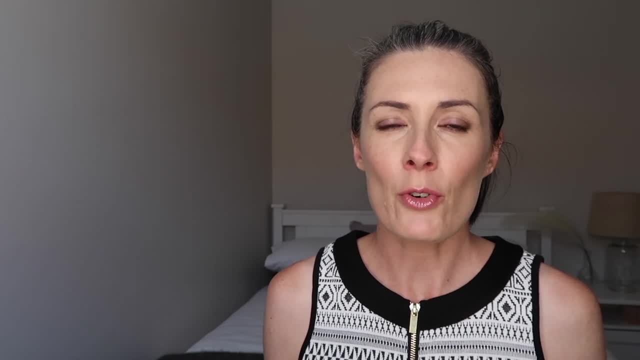 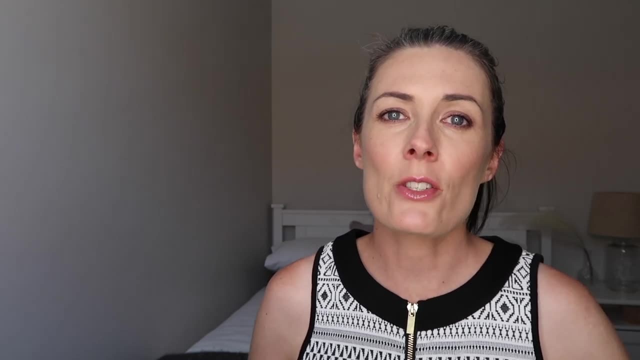 I know a lot of you also watch her channel, And so you may have already heard her talk about her course or heard me talk about it in my previous videos. Nuria does publish children's books, And so she created a course on how she does it, And in fact, she just actually won an award for one of 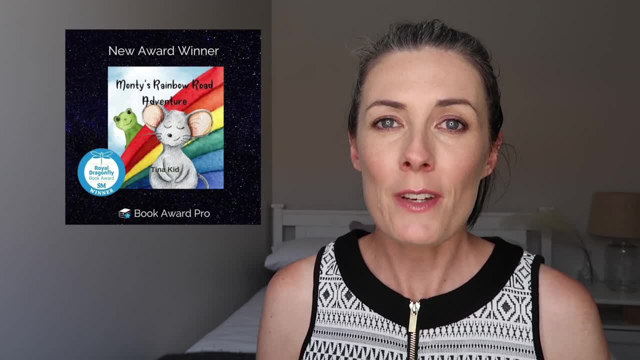 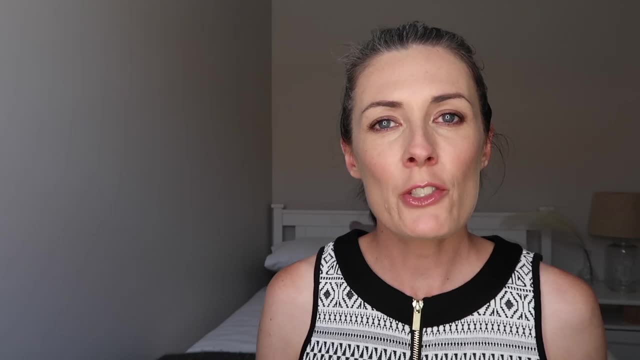 her books, which is called Monty's Rainbow Road Adventure, which is a book All about learning colors. So congrats, Nuria, It is well-deserved. But my point is, if you are interested in taking her course, you are going to be learning from somebody who publishes books. 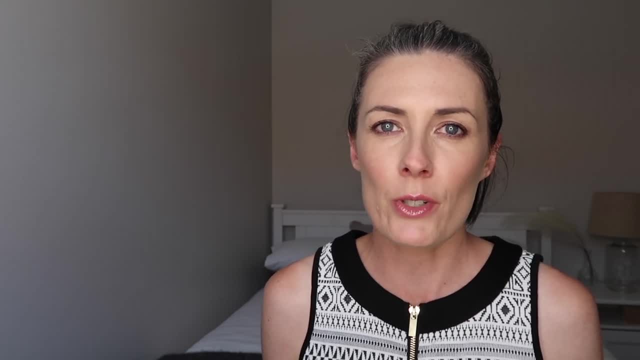 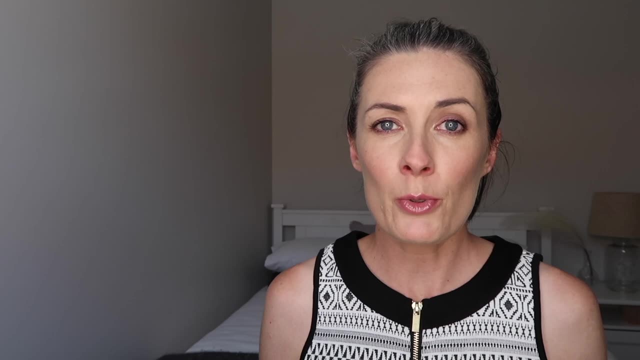 herself and knows what she's talking about when creating these kinds of books. I do have links to her course in the description below if you want to find out more information about it. It is an extremely affordable course in my opinion, especially considering the amount of content. 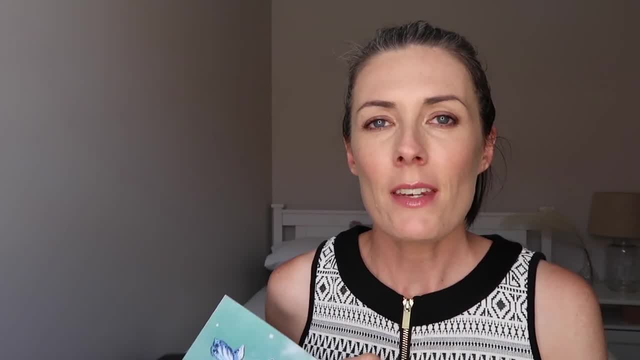 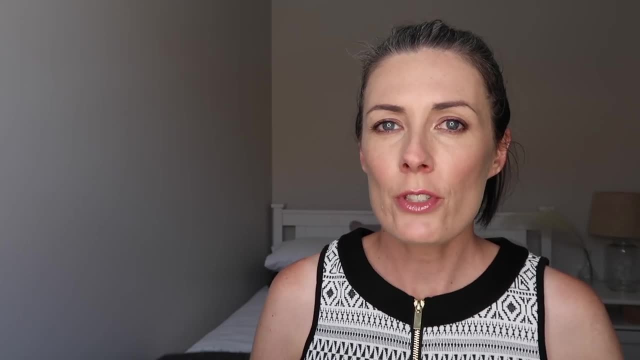 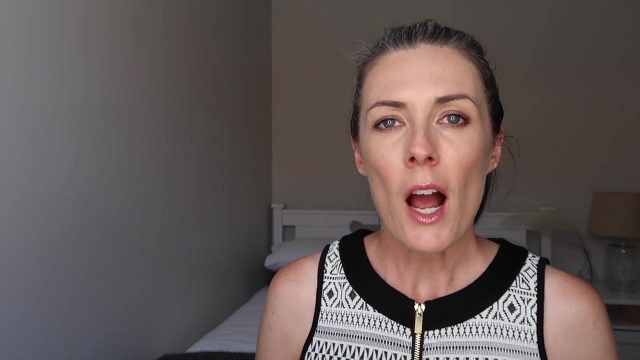 that is in there, And so just going back to my book Now, I did do a soft launch, I would say, of this book, a very small experimental soft launch. I did do some paid promotions on some book promo websites and email lists for when the book went live I also sent out some advanced 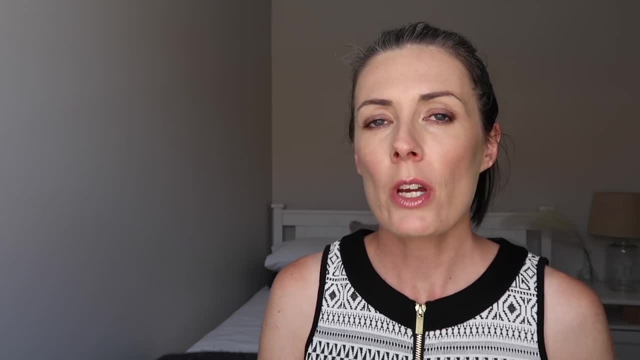 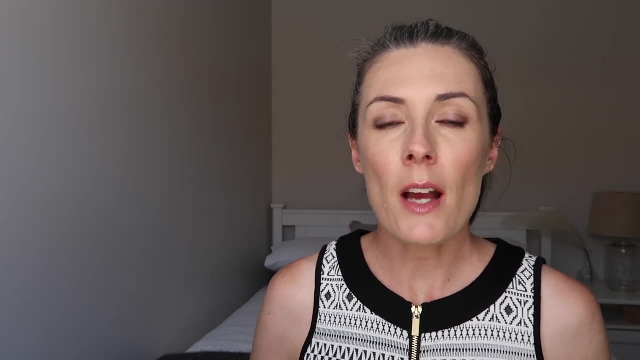 copies of the book, some digital copies of the book, to people who were interested in reviewing books in general, And when they said they were interested in reviewing mine, I was happy to send them a digital copy in the hopes that they would leave me a review when the book went live And I 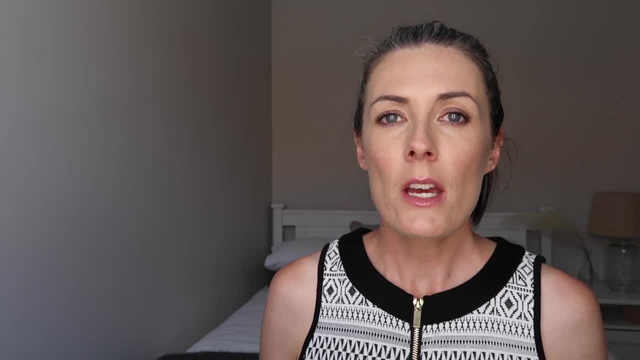 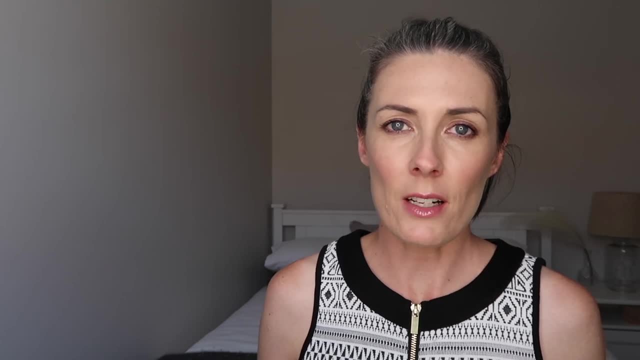 also sent out some reviews right out of the gate, some sales right out of the gate, to help the Amazon algorithm decide or determine whether my book was going to be popular, whether it was going to sell, whether people were going to like it, which would, in turn make them hopefully push it. 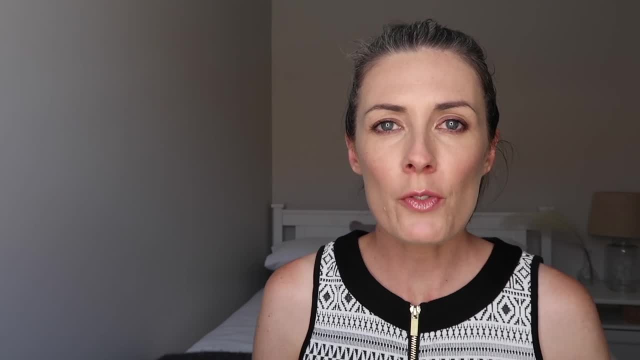 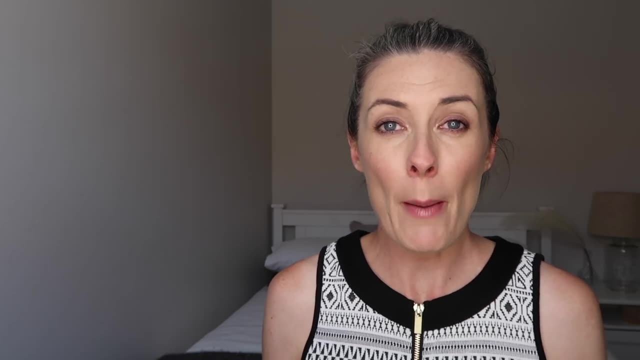 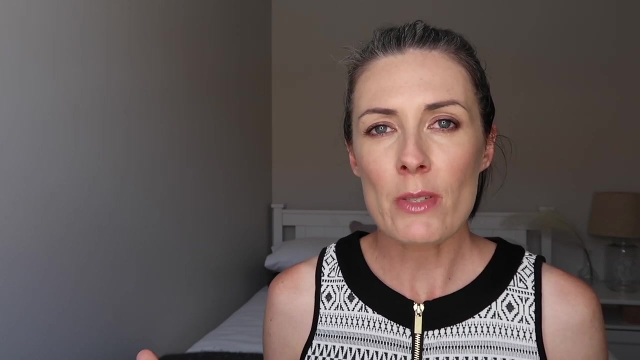 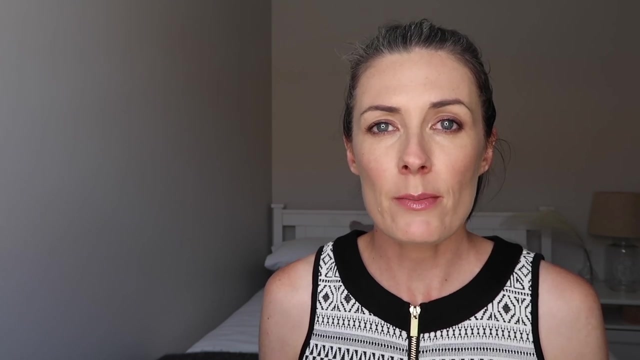 in the search results to their customers. Now I have done a few videos recently where I talk about the importance of that first week, or the first couple of weeks of a book being live on Amazon and what happens in those first few days. I also did create a Kindle version of the book and it wasn't my original plan to create one, and 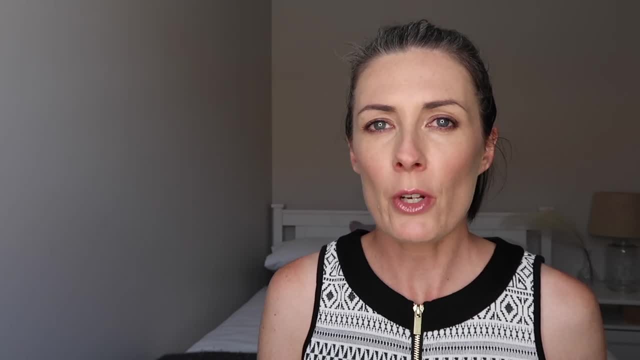 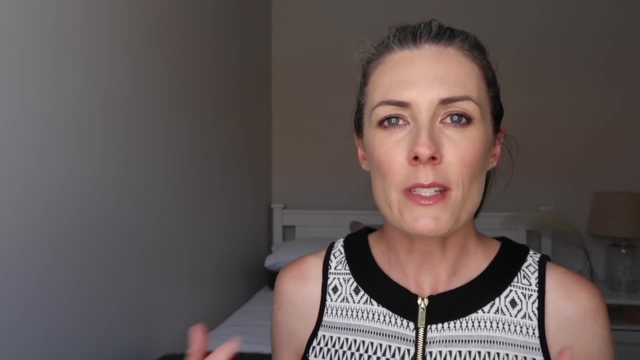 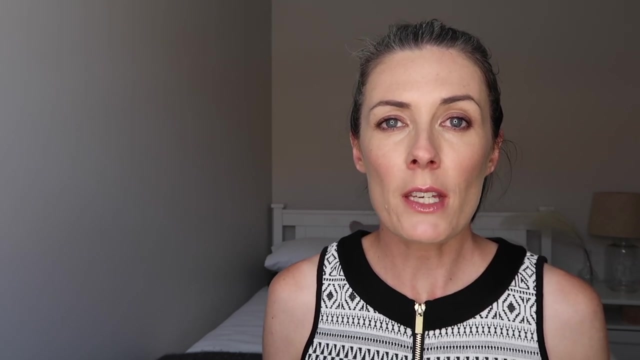 selling the Kindle version of the book isn't really my priority because I don't feel like children's picture books are really made for Kindle. They're made to be a paperback where you sit and read them with your child. as a parent, I did create a Kindle version of the book because I did want to do a free giveaway and be able to 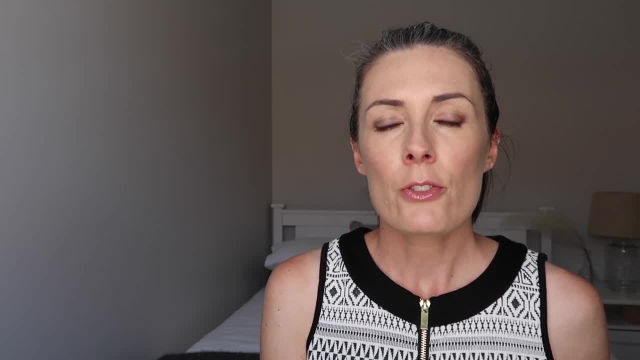 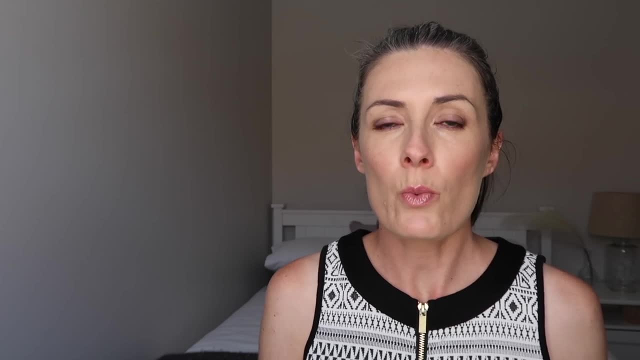 send that free copy of the book to people to generate as many sales or downloads, I guess in order to get reviews as soon as the book was live on Amazon. And aside from that, I have run no further promotions and have done no advertising. 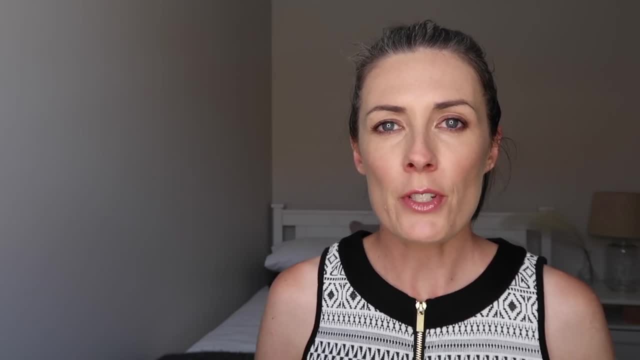 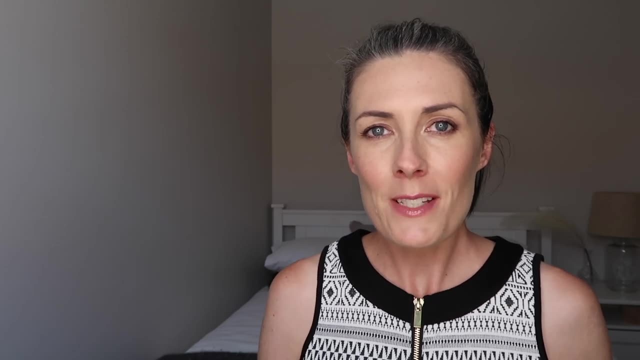 at all for this book. So I made the book live on the 1st of November 2021 and since then, up to today, the day that I'm filming this video, which is the 13th of December, I have sold a total of 649 Kindle. 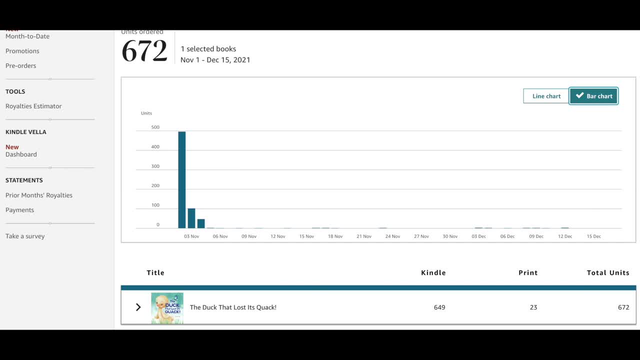 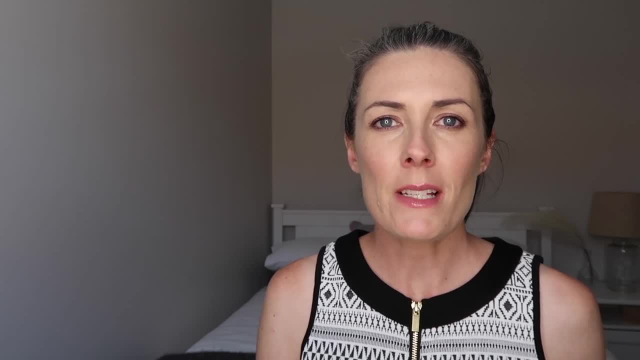 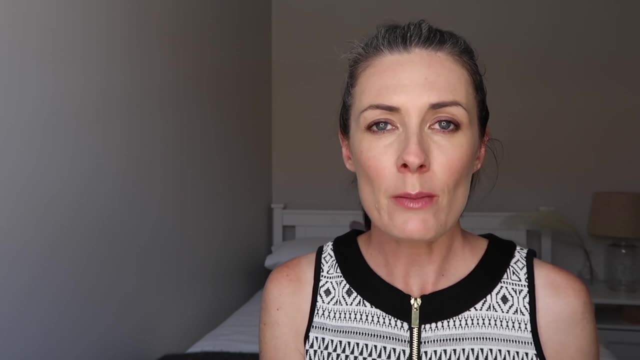 copies- majority of those were free copies- 23 paperbacks and have received 3,441 KNEP reads, which is basically the Kindle Unlimited subscription, where Amazon subscribers who are subscribed to Kindle Unlimited can read books for free or as part of their subscription, in the sense. that they don't have to go buy the book. They can read it through their Kindle Unlimited account and authors get paid per page read. So having a children's book isn't going to generate much money through that side of the business, because that one generally works by volume. The bigger the book, the more page reads you're going to get and you're going to get paid more. So that's just a very small part of it that gets added on. But for children's books, ideally, you're going to be wanting to be selling mainly paperbacks. 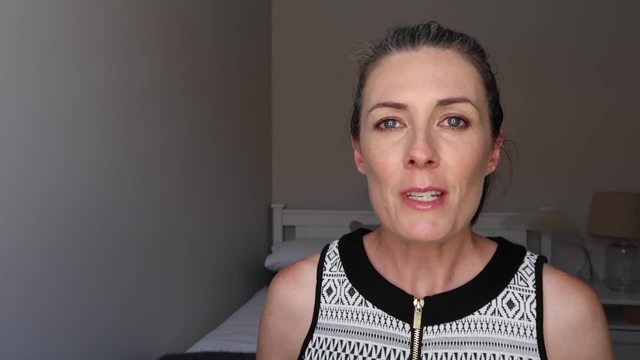 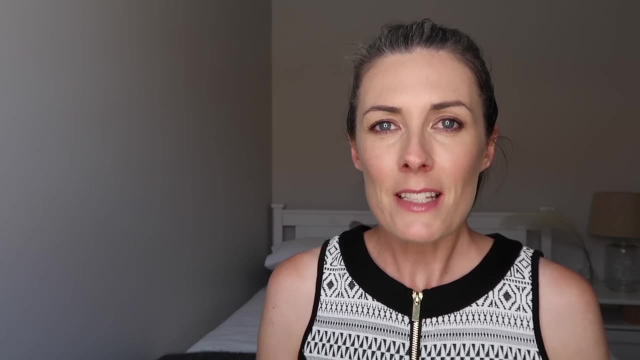 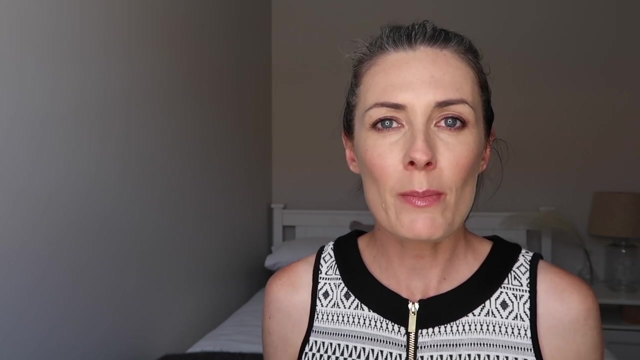 So at this point I've made about $100 in total. So that's pretty much it from this book. Now, that's nothing to write home about, It's nothing that I'm going to be able to retire on, but it is my first children's picture book that I've created, and I do have plans to make more. 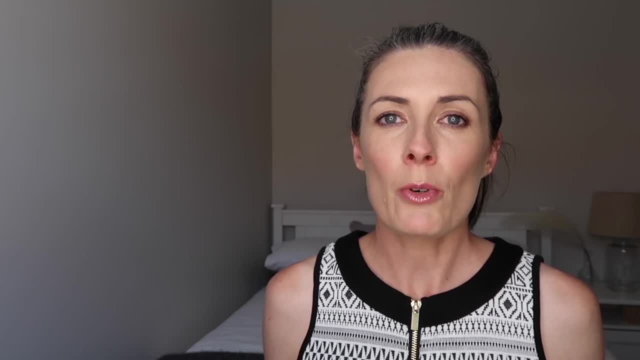 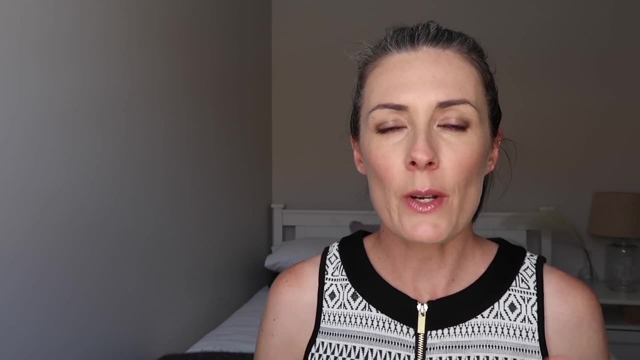 And that's a book that is pretty much selling from day one, with almost no promotion at all. once it went live on Amazon, The sales are increasing each day as well, compared to when it first went live, So at this point it is selling multiple books a day, which I'm really happy about. As time goes on, reviews build and more people provide their feedback about it, then hopefully the sales will just continue to increase, Also with the addition of more books added to it, more children's books added to it. that can also help increase sales as well. When someone buys one book, sees that you've got others and they liked your first one, they may go off and buy other books that you have as well, But for now I just want to start looking ahead and start creating the next one. 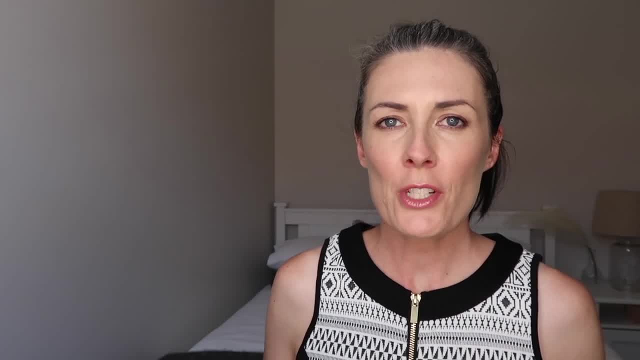 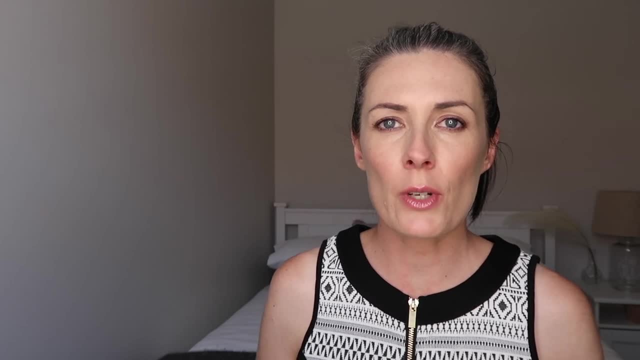 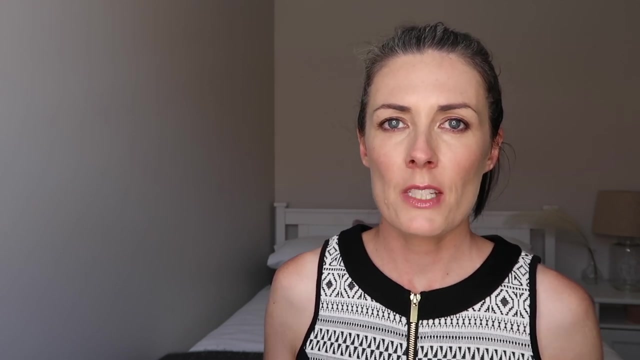 Enough about all that. How exactly did I do all this? Well, firstly, as I said, I did take Nuria's book creator course, And what's really great about that particular course is it teaches you how to create the whole book without hiring expensive illustrators or editors and all that kind of stuff. 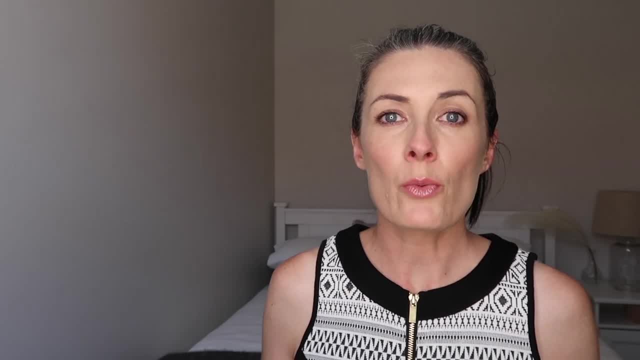 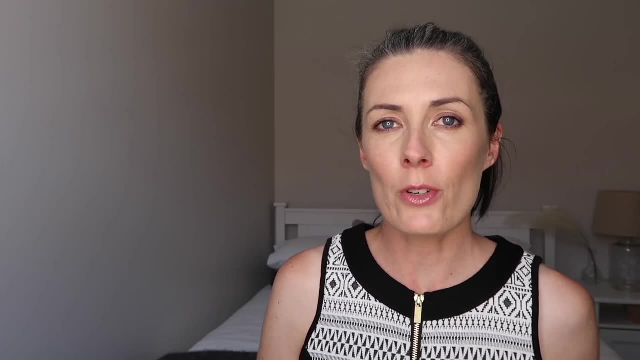 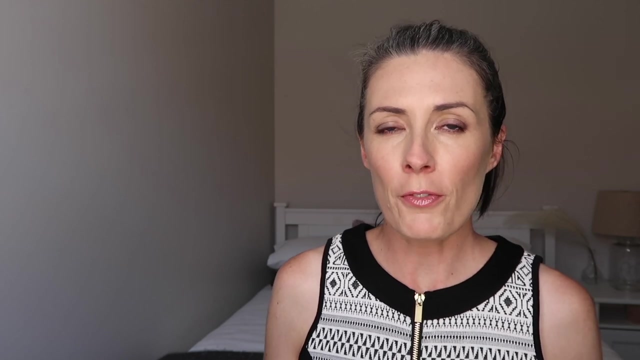 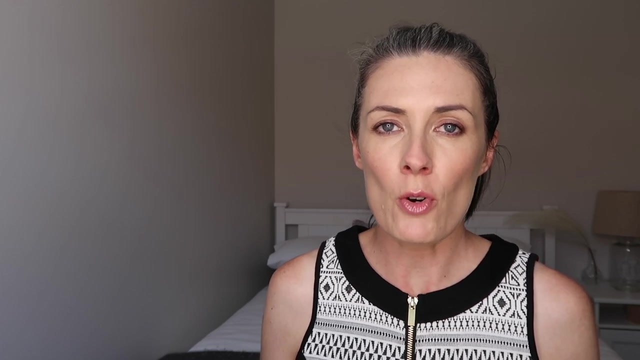 So after completing the course, my first step was writing the book. Now, I did have an idea for a story lurking about in my head for a little while before taking the course, But you will get ideas on how to do that, How to come up with story ideas and how to find the more profitable kind of stories in terms of finding what kinds of stories parents are actually searching for on Amazon. 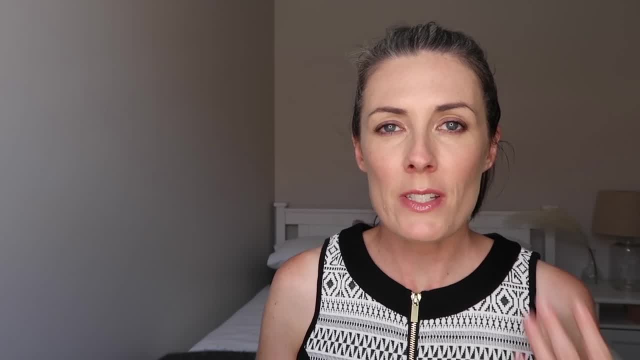 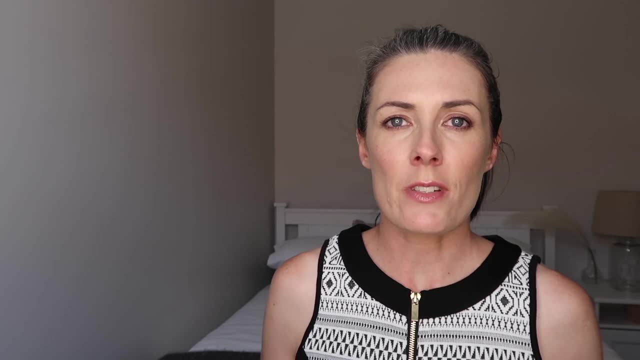 And I decided to write a rhyming story because, personally, those are my favorite kinds of books to read when I'm reading books to my little girl. From there it was time to illustrate the book, And this part I was really, really nervous about. 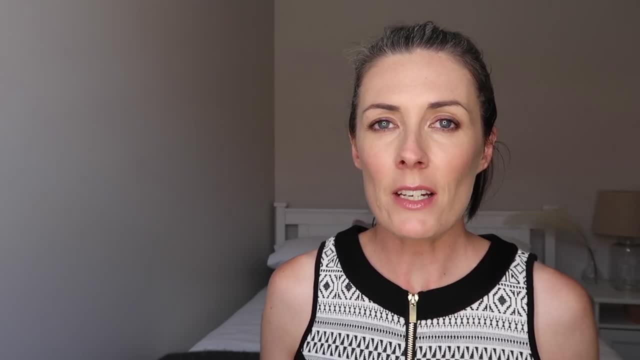 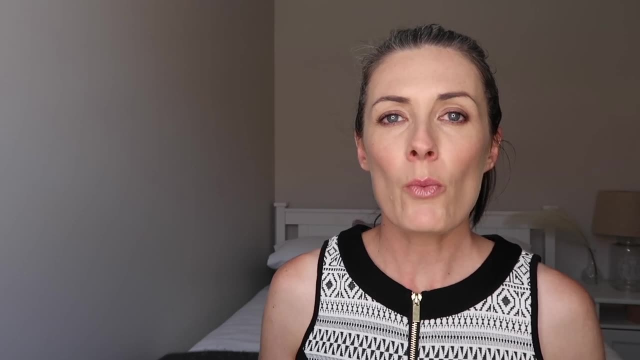 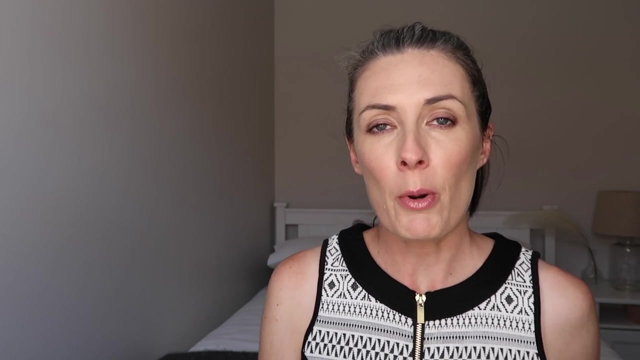 And this part I was really, really nervous about. Like I said, I've never illustrated or done any kind of illustrations before and I wanted it to look professional and match the idea that I had in my head and I wanted it to be able to compete, be on par with all those other books on Amazon that are professionally. 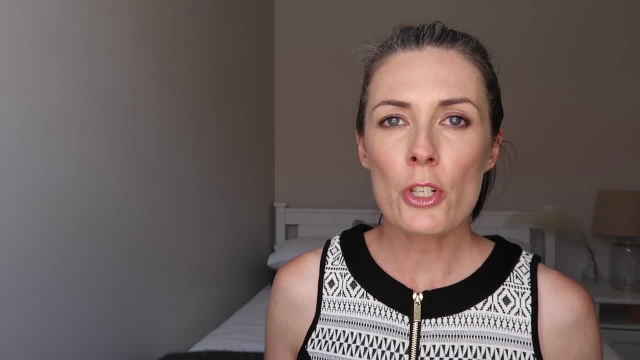 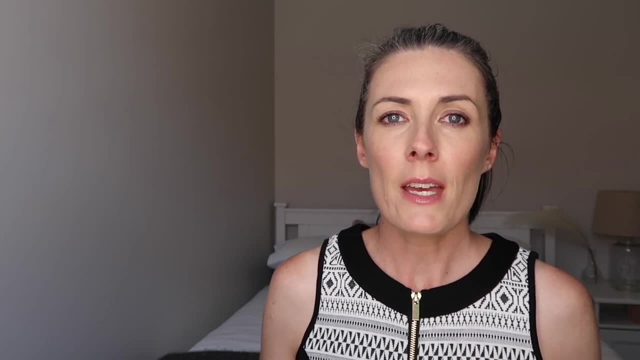 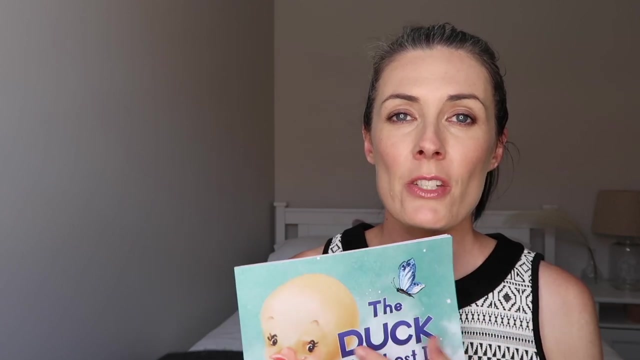 published and are professionally illustrated. So after watching the modules in the course about the illustrating of the book, I was able to find some really beautiful illustrations and I ended up going for a watercolour style that I felt matched my story and this little duck here, this is the main character of my 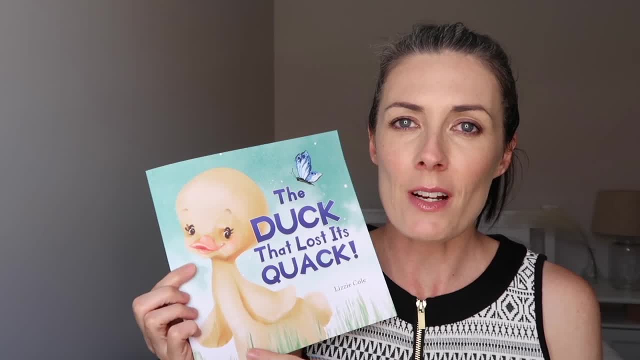 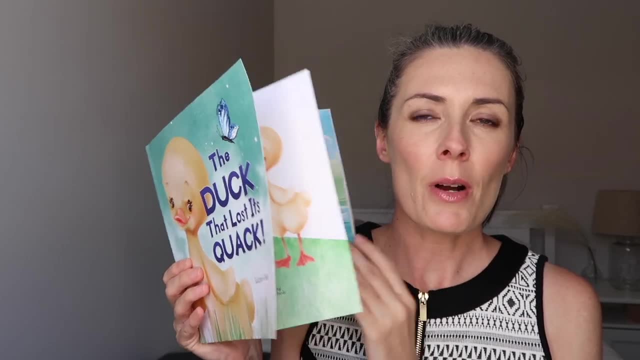 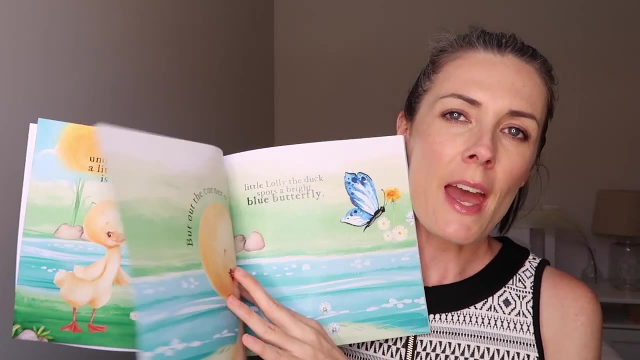 story. That was the first illustration that I found. I looked for the duck first and her name is Lolly the duck, And all of these pages in this book. they are made up of multiple illustrations, So some of these I purchased. Some of these I took from the Canva Pro account, where you get access to their graphics and 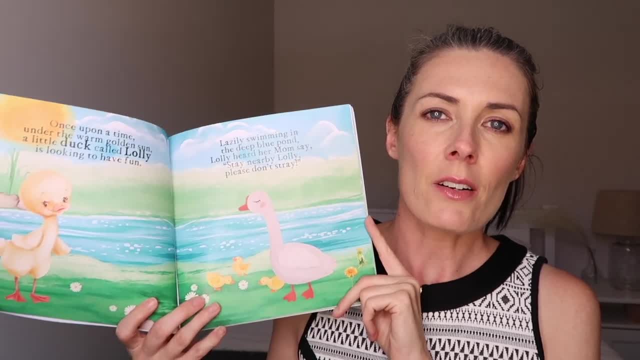 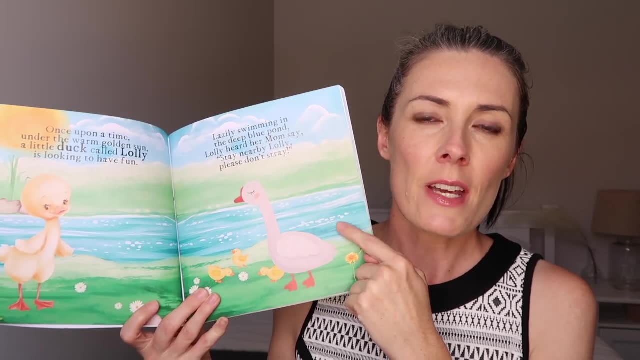 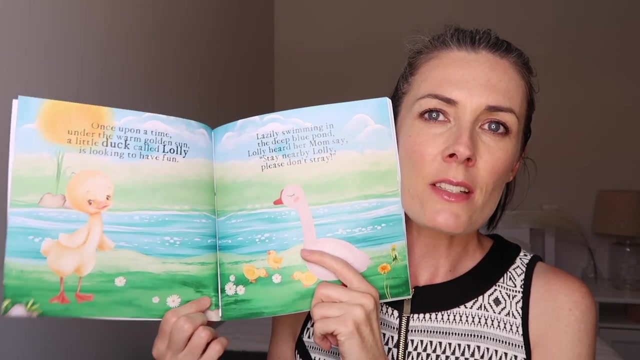 I just layered them all together like this. Now it's not as hard as it seems. I basically started with this background, which I purchased. I then added things like these clouds which I took from Canva, all these little flowers and little ducks and stones and leaves and the sun. 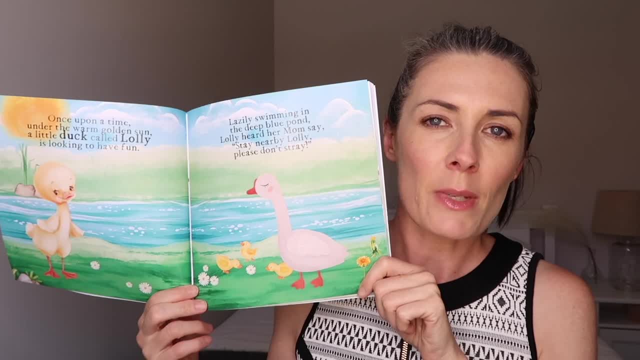 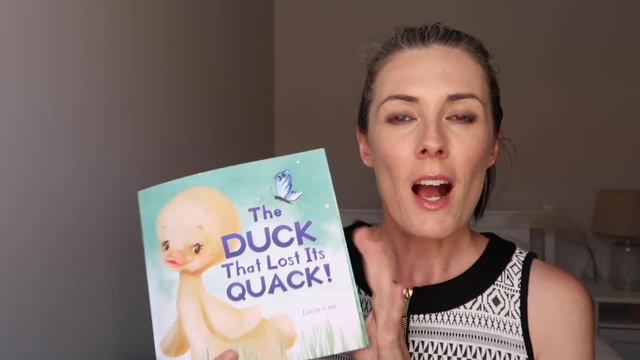 These are all stuff, Separate graphic elements, mostly taken from Canva, the Pro account of Canva, some taken from the illustration packs that I purchased. And, just talking about Canva, I actually created this whole book in Canva. I do recommend the Pro version of Canva. 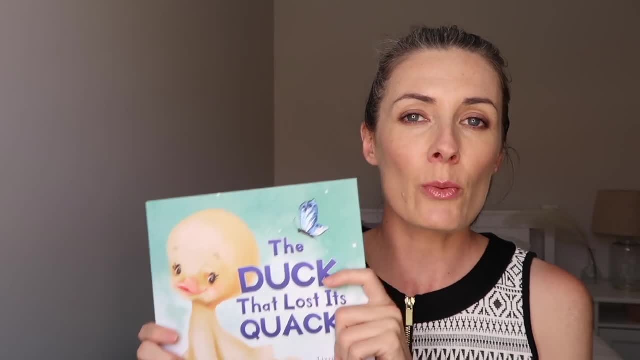 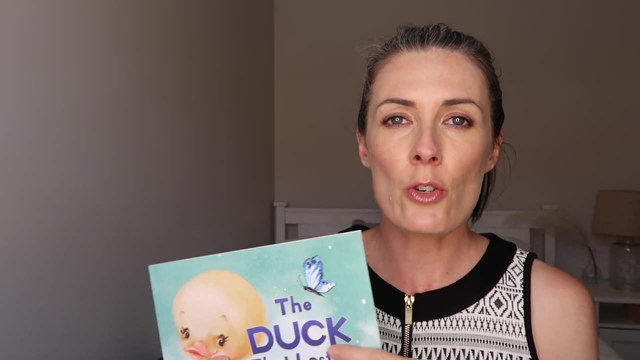 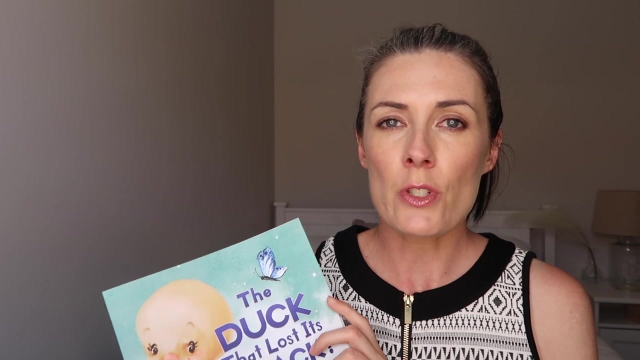 I really do feel, especially after making this book. I really feel that the graphic elements you get access to in the Pro version are just so much a better quality and you have such a bigger range to choose from When you are creating something as detailed as a children's book. 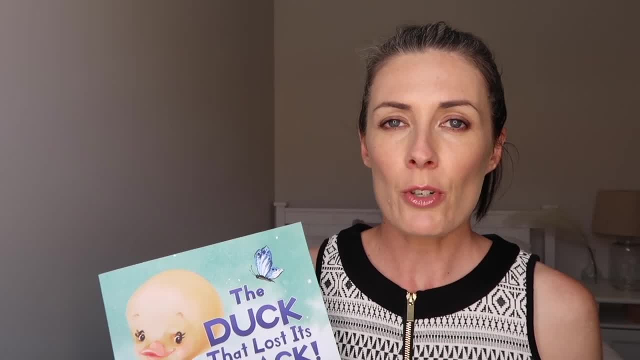 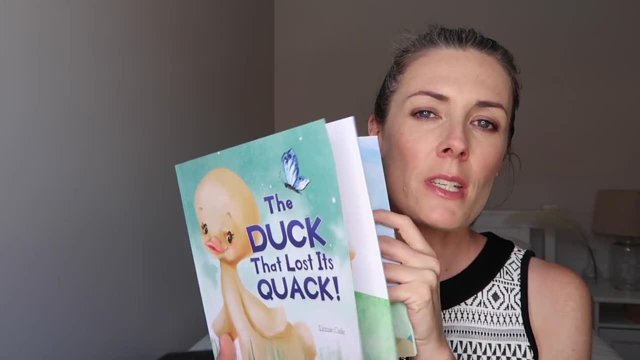 But in saying that if you cannot get access to the Pro version, if it's just not in your budget, it is fine, You will be able to get by with the free version. Now the font inside that I used this particular font I also purchased from a stock font website. 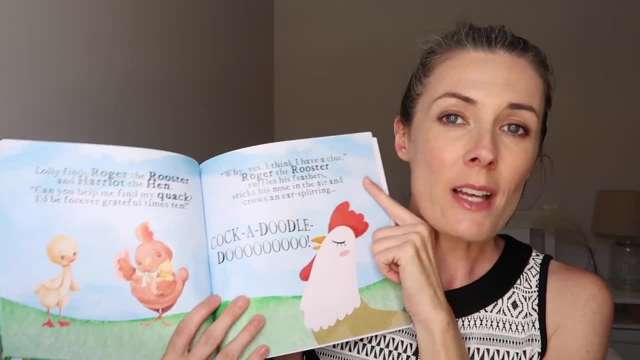 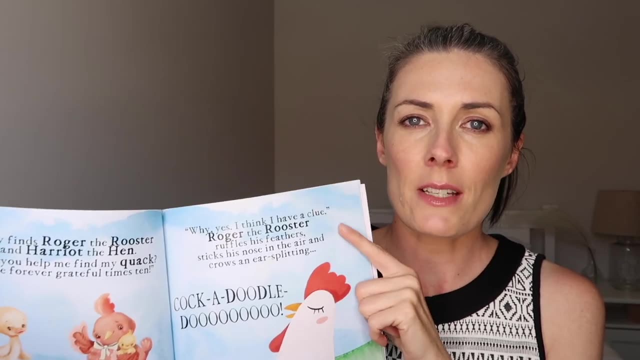 I actually think I got that from Creative Market because I had a really specific idea in mind of what I wanted my font to look like. But again, Canva has: You can use fonts that you have access to, free ones and more within the Pro version. 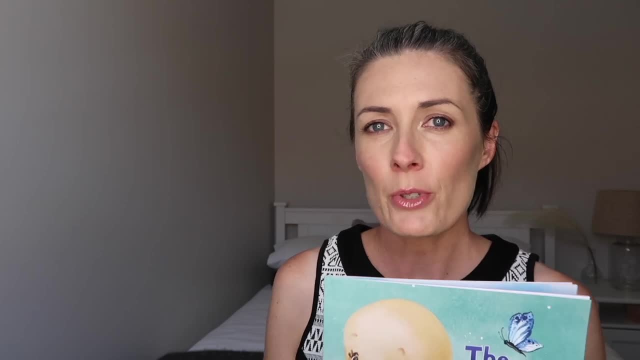 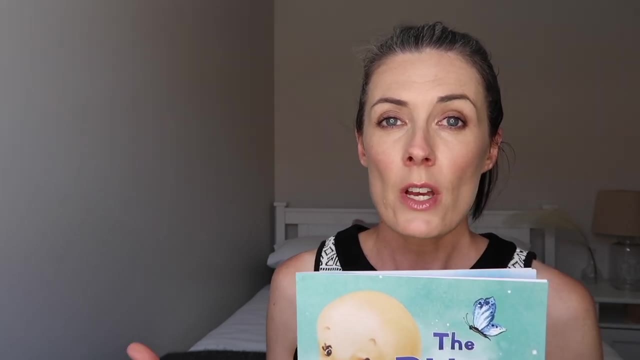 if you just want to use the elements in Canva Now also, you don't have to create the book in Canva. That's just what I ended up using. You can use whatever graphic design program that you normally use. You can even create it in Microsoft PowerPoint. 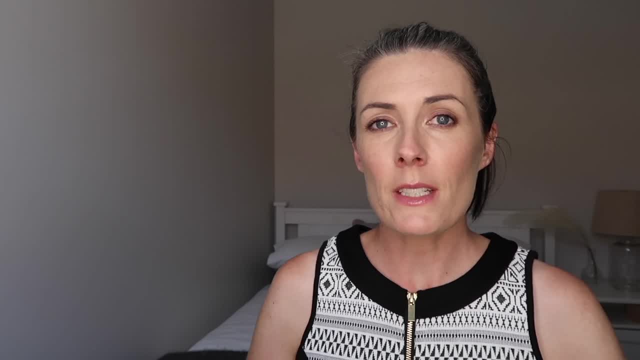 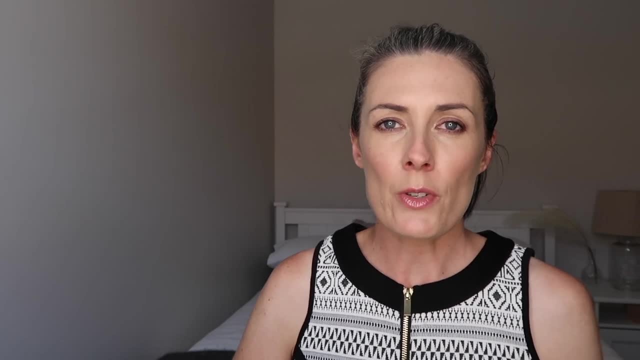 That would work really well too. To give you an idea of what I spent on the illustrations and also the font, I spent around $50 in total for all the illustrations that I purchased. Then, of course, if you have the book, you can get the book in Canva. Of course, if you have the Canva Pro account, you have a Canva monthly subscription that you need to pay for, But it is just a very small amount when you compare with how much you would be spending for a professional illustrator, which a lot of times can run into the thousands of dollars. 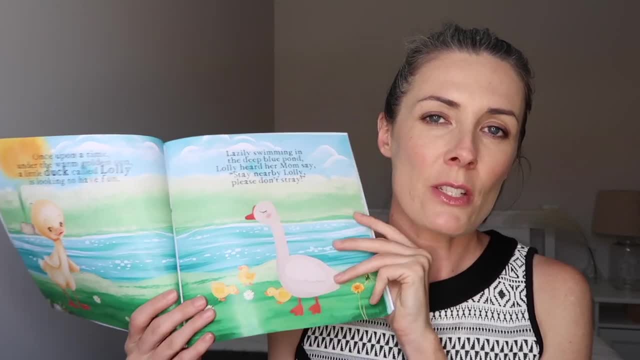 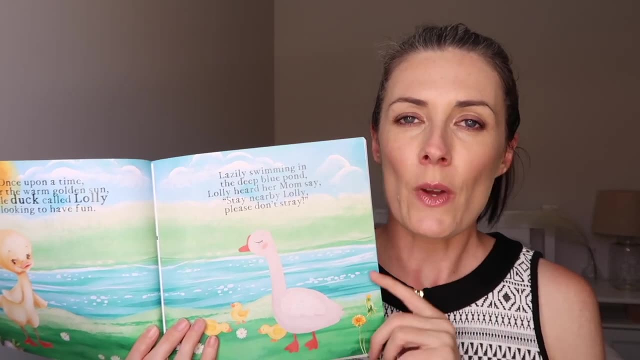 And so basically, once I had sort of made these sort of pages where I added all the elements, I just kept playing with it and just tweaking, moving things around, seeing how I liked, whether everything fitted together. I was happy with how the pages looked. 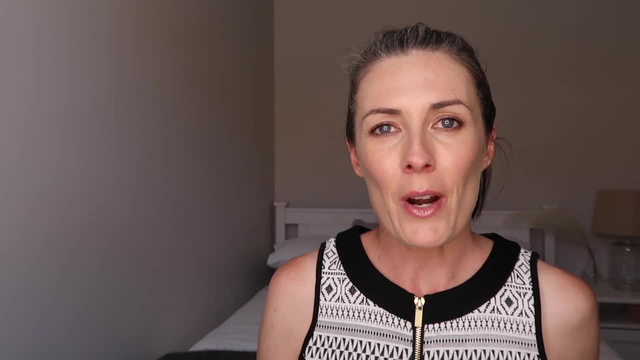 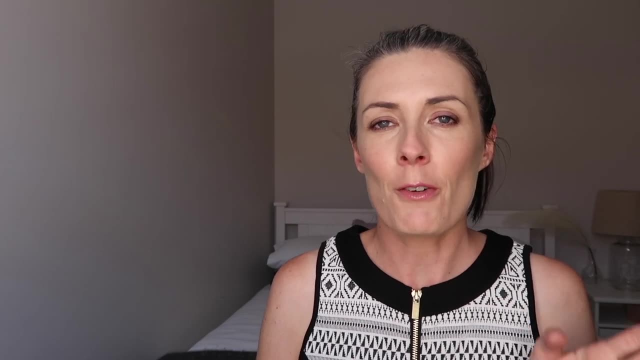 I was happy with how the pages looked. I was happy with how the page came out. Now it did get to a point where I had to say to myself: enough is enough. You could just spend forever tweaking this, moving elements around, adjusting fonts and 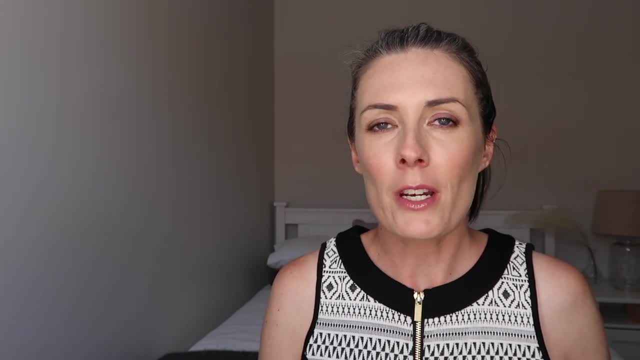 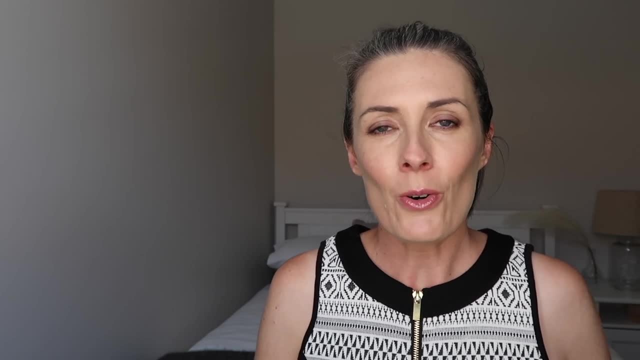 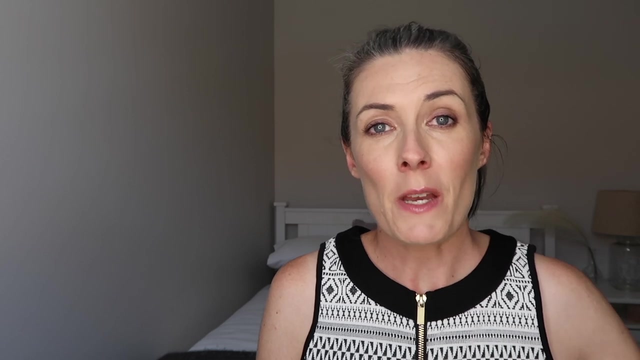 things like that. Sometimes I do fall into that trap of trying to make something perfect and then end up never finishing it. So if you're somebody like that who tends to get caught in that trap of I need to make this perfect before I can get it out there, you have to get to a point where done is better. 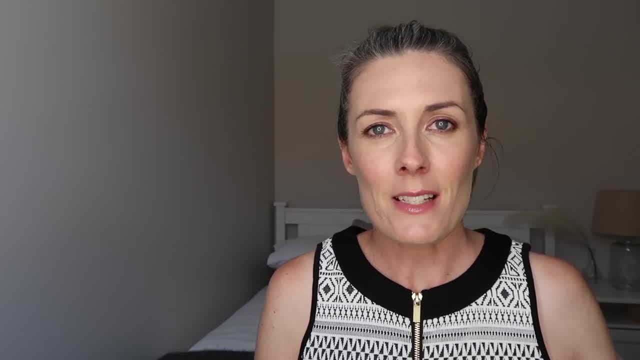 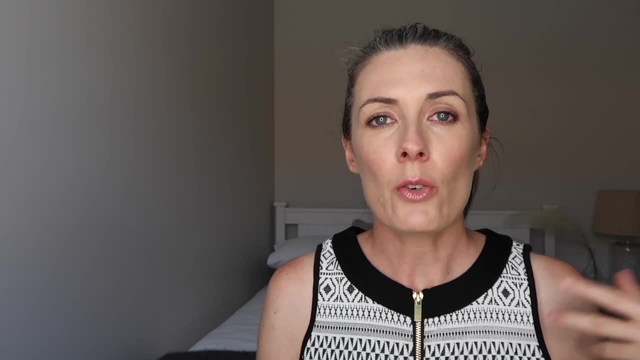 than perfect. Just get it out, Get it done, Get it live, Get it selling, And if you really feel the need to edit or adjust things later on, you can. You can edit it, You can re-upload it, You can adjust your images, re-upload the book. 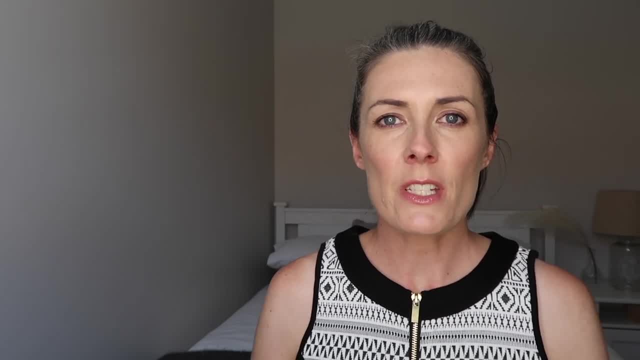 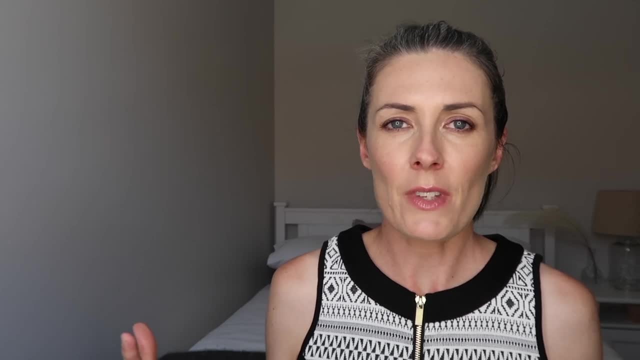 It's totally fine. Now, also, if you have zero experience with graphic design or even just using things like the free version of Canva, creating something very simple. there is a whole massive module in Nuria's course. There is a whole massive module in Nuria's course. 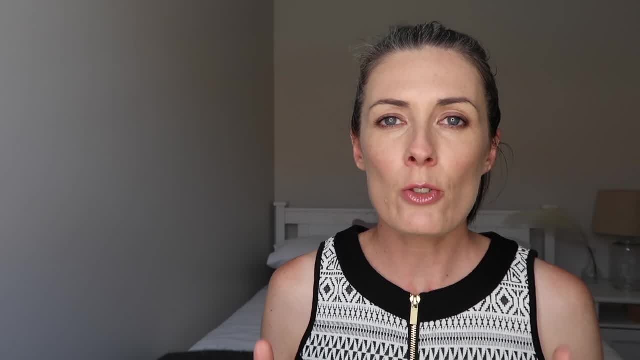 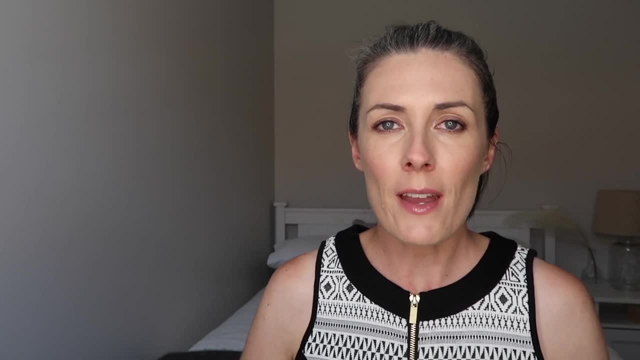 Where she has a video or a module for every single page of her children's book. Within her course, you follow her making her children's book and she shows you every single page that she creates and how she does it and how to create the page in terms of laying. 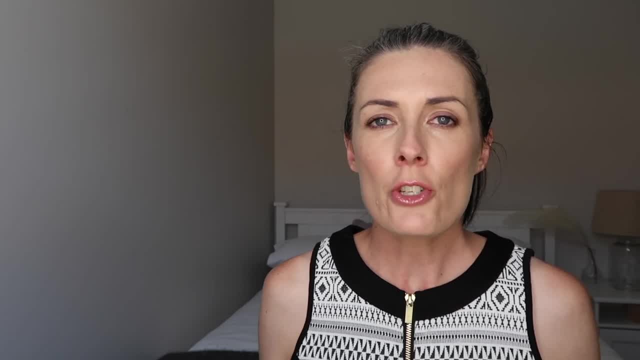 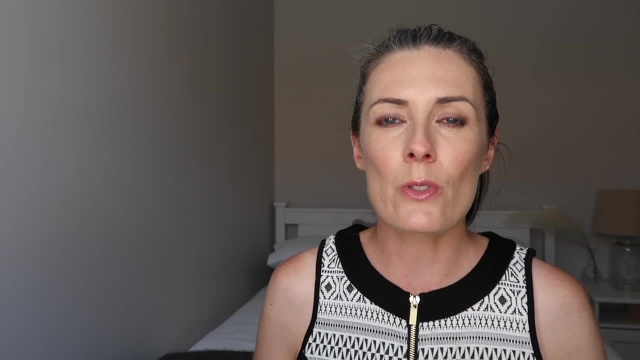 it out where certain design elements should go and how you should lay it out to look appealing to both parents and children. So if you have zero graphic design or illustration skills, don't worry, There is something there. There is something in there for anyone, even those who are total beginners. 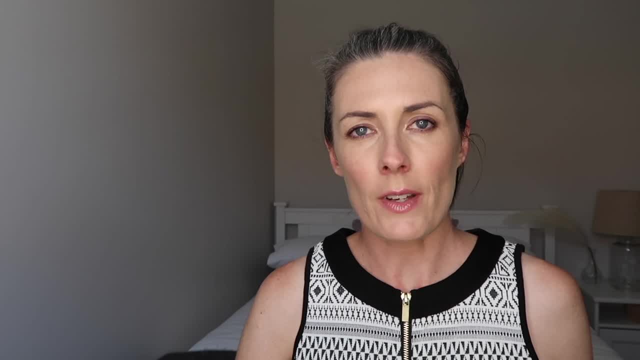 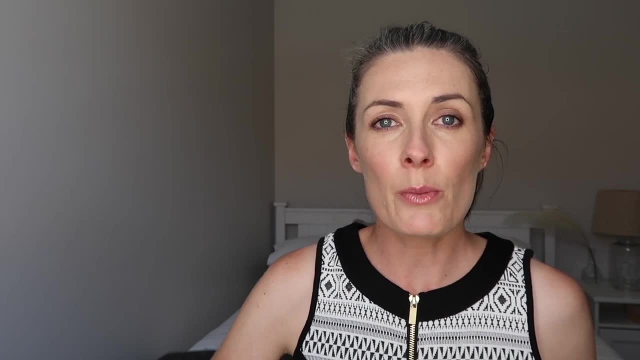 So once I had created my interior pages, I then started to work on the cover, And the cover I wanted to keep sort of minimalistic, sort of simple, also matched the interior's style of the book, which has that watercolor style and showing off the main character of 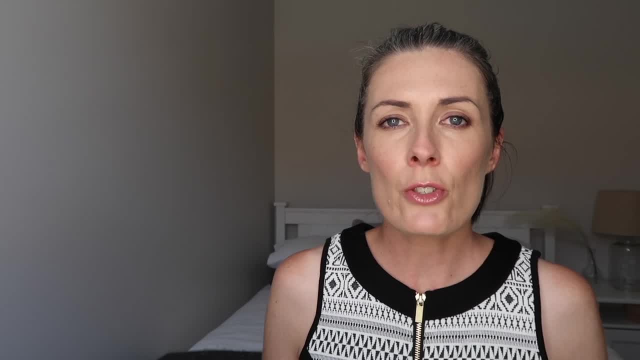 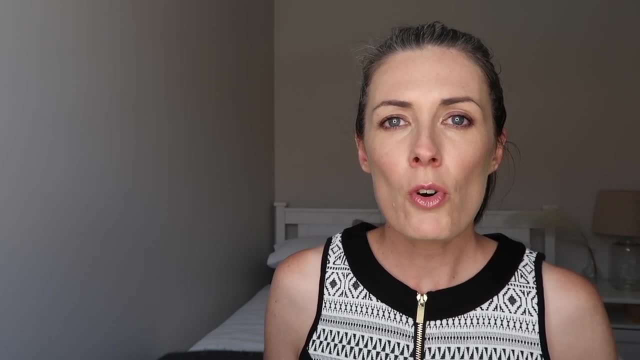 the book. Something that I did a lot of was I went onto Amazon and I looked through all the children's picture books and looked at particularly the best selling books. I looked at what their covers looked like. What kind of fonts did they use? 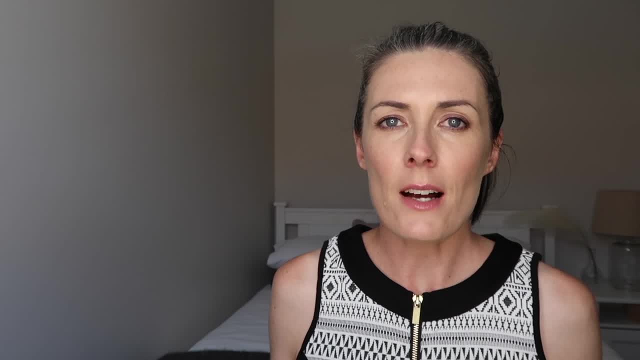 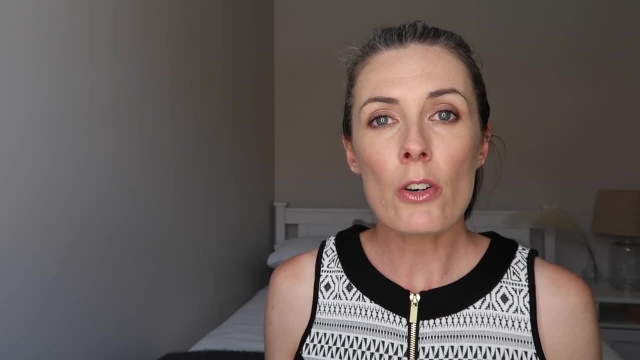 What kind of colors did they use? How were their covers laid out? What sort of elements did they have on the covers? I wanted my cover to fit in with my genre so that it looked like it belonged, but I want it to stand out enough so that it is noticeable within the sea of hundreds of other. 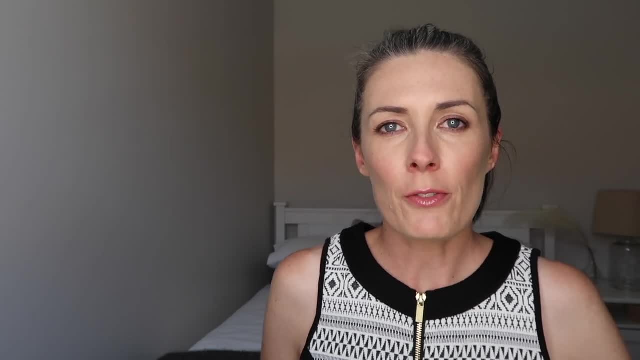 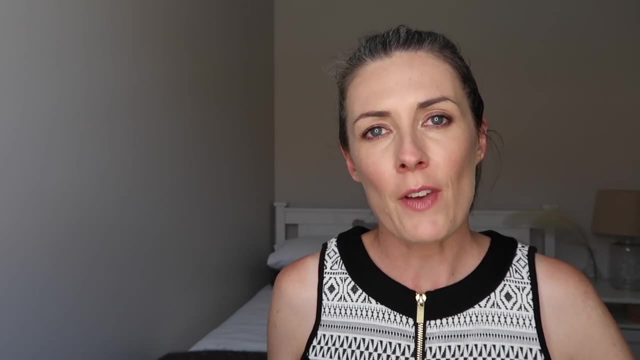 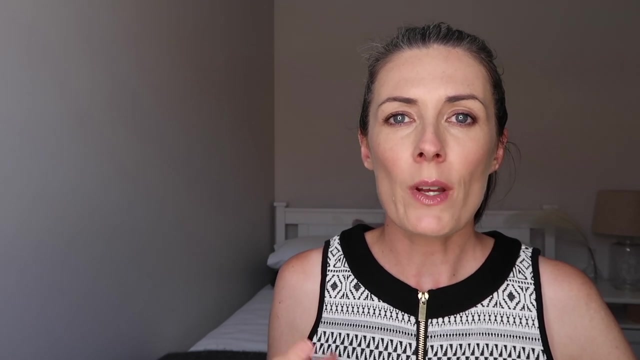 thumbnails on Amazon. I also experimented with different fonts for the cover, which I did want to make different to the font that I used inside, And I tried a few different ones till I found the one that I liked the most. I wanted the cover to be visible enough and clear enough so that when someone's on Amazon. 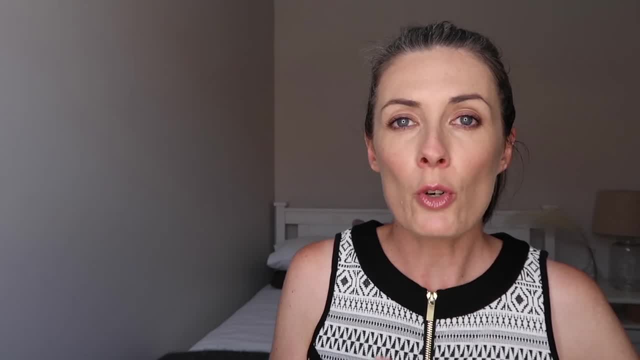 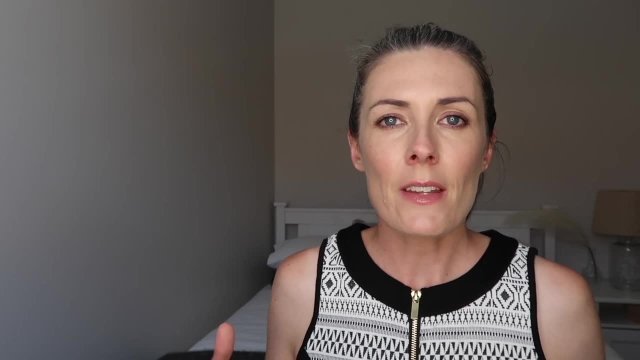 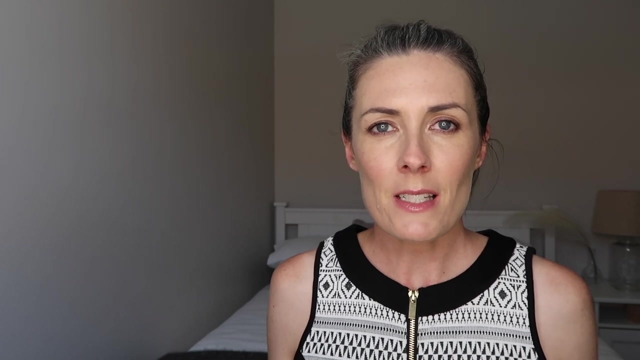 looking at a thumbnail sized image of your book, they can clearly see the graphics and the fonts and the title of the book and everything like that. So I didn't want to clutter the cover up with so many graphics that you couldn't see the font, you couldn't see the title and it would just be a disaster if, when your book is that, 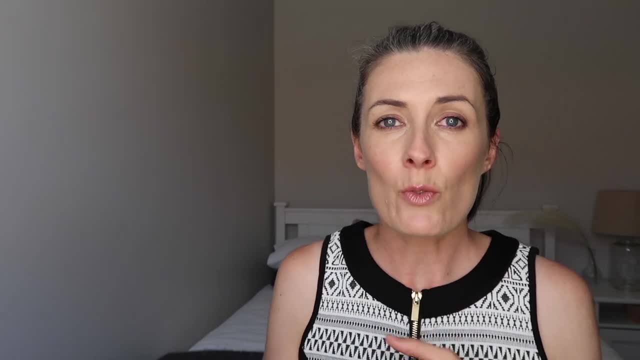 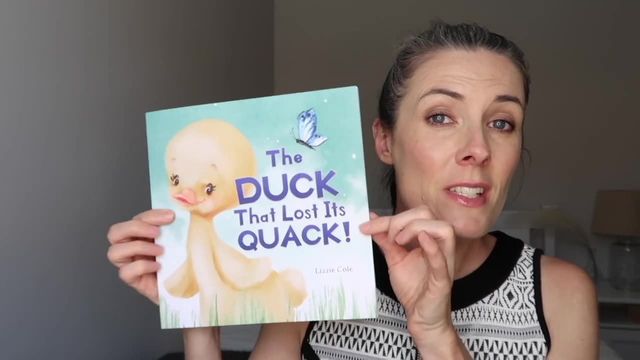 really small, thumbnail sized image that a customer can't even read the title of your book. So that's something that's really important. you have to remember that when someone's on Amazon, they're not looking at this size of a book on their website. 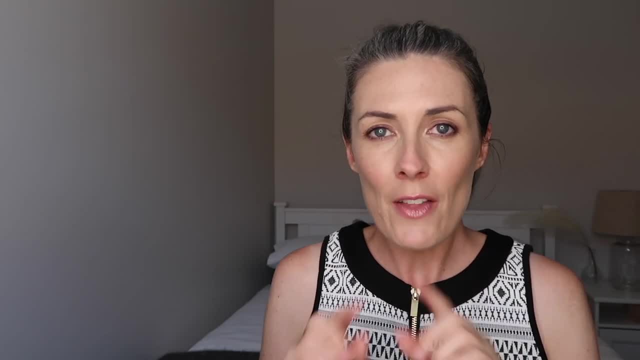 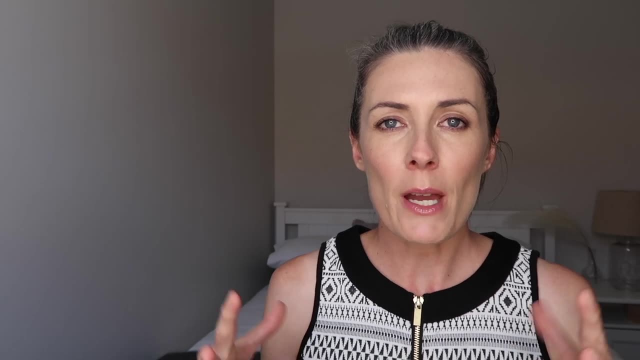 They're looking at this tiny little square surrounded by hundreds of other tiny little squares, and your customer needs to see what the book's about, what the title is, and be able to clearly read it in that tiny, thumbnail sized image. Once I had done all the graphics side of things, 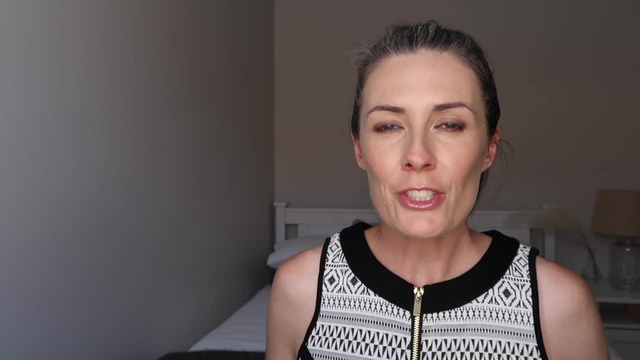 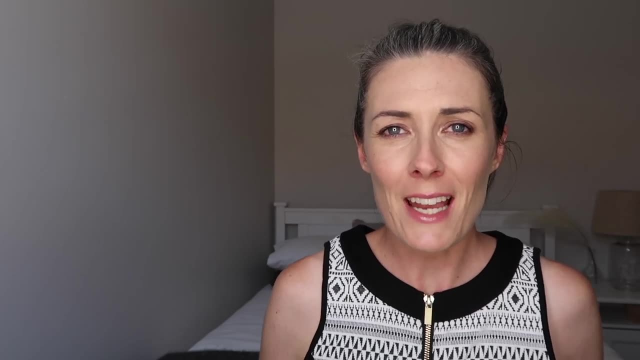 I then needed to write the blurb for my book, which honestly, I think was actually so much harder than writing the actual book. The blurb, I think, took me two or three days to actually get to how I was happy with it. So the blurb is this part on the back of your book which helps to just summarize what your 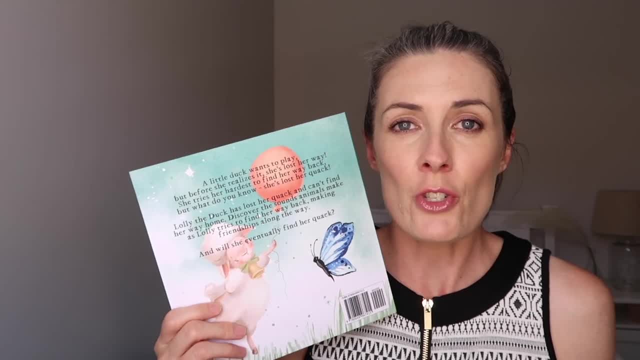 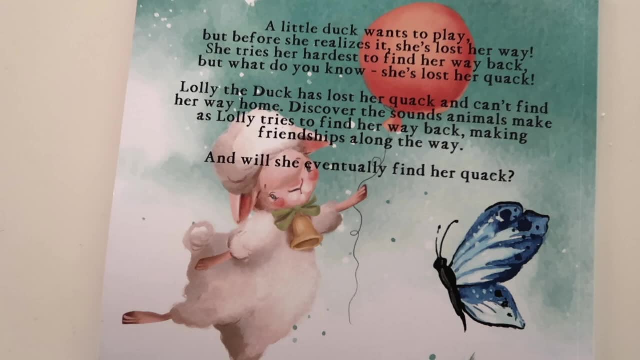 story is about and hopefully entice a customer to purchase your book based on your blurb, And my blurb currently reads: a little duck wants to play, but before she realized it, she's lost her way. She tries her hardest to find her way back. 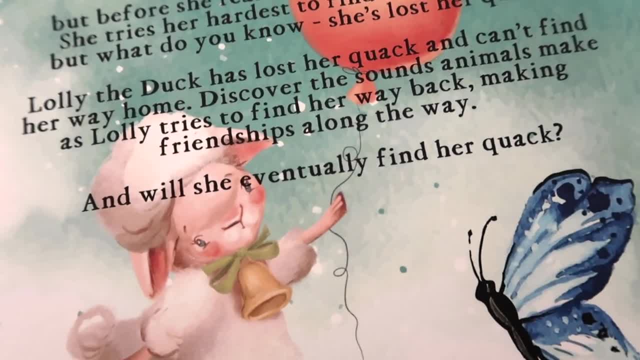 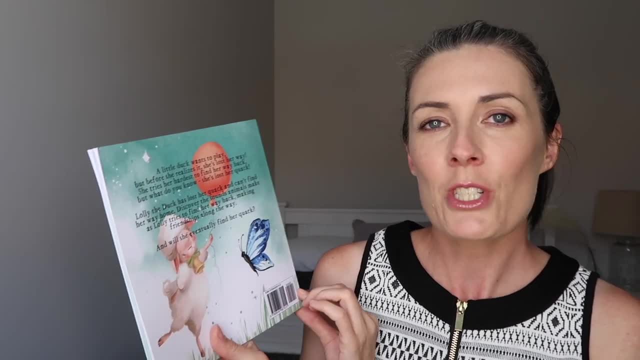 But what do you know? She's lost her quack. Lolly the duck has lost her quack and can't find her way home. Discover the sounds animals make as Lolly tries to find her way back, making friendships along the way. 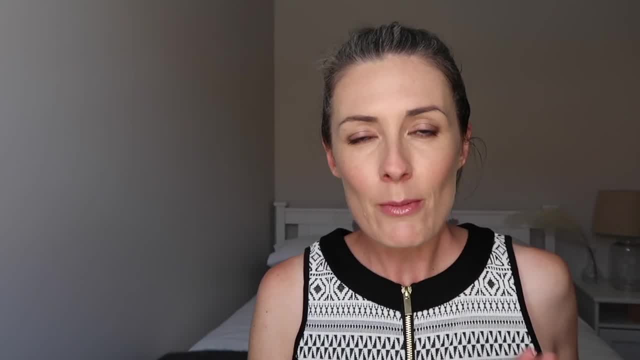 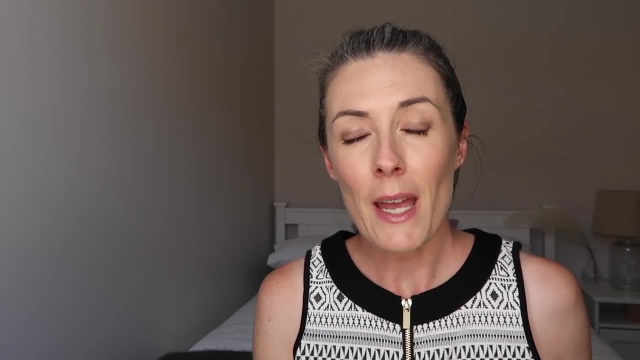 And will she eventually find her quack? And so that was what I ended up going with as my blurb. So once I had created my blurb, I also then had to create my description, which was going to go on the Amazon sales page for the book listing. 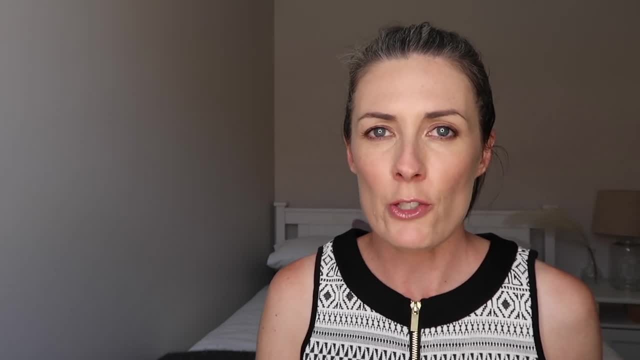 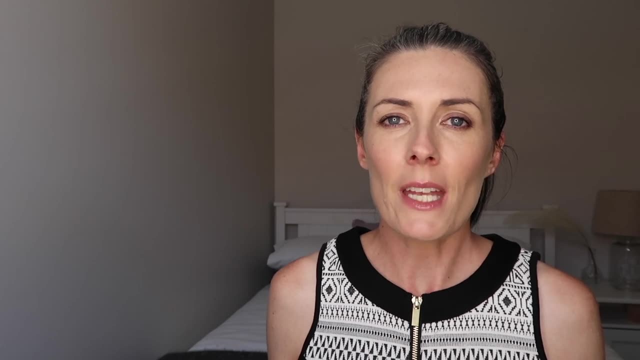 And I also created things like my bio to go on my author central page And then I uploaded the book. I had all the elements I needed, And uploading the book is basically the same process as uploading any other kind of book. So if you have experience with low content books or even high content books in different 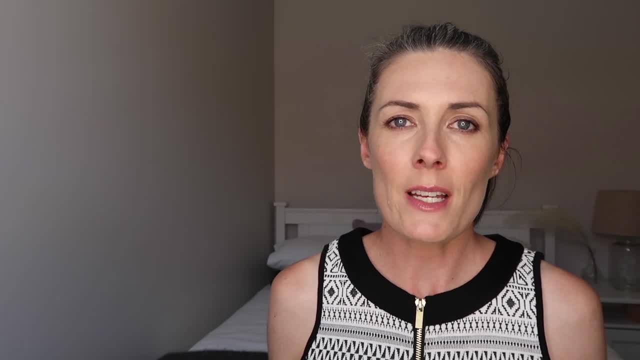 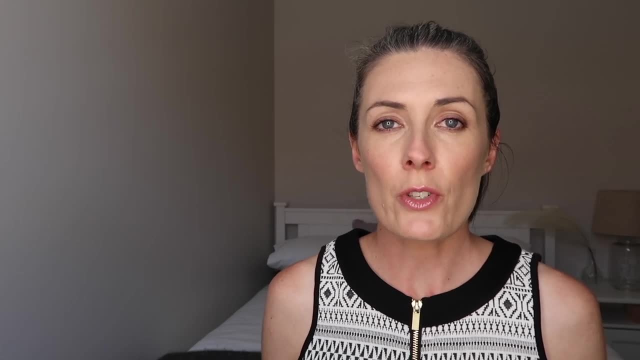 genre than children's books, then you'll be familiar with this process. It's the same. It doesn't matter what kind of book that you're uploading, And once it was submitted, it was only a few hours and it was approved. So the approval time, or the wait time to get your book reviewed and approved, is so much. 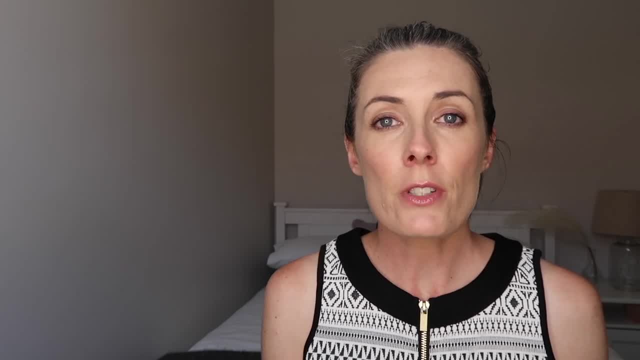 faster with actual storybooks or high content books, So I'm going to go ahead and create a new one. So in my case, I have five books that I'm uploading every day and I'll be uploading the book every day. So if you're making books with high content books, then it is with low content books. 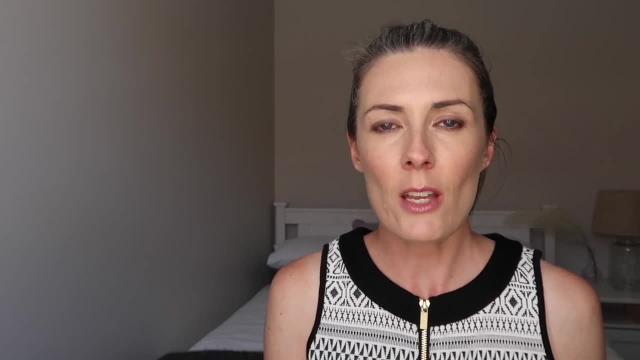 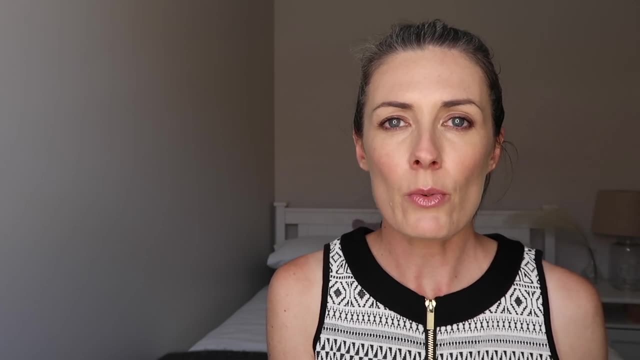 When you're making things like notebooks, journals, coloring books and things like that, it just seems to take forever to get reviewed, And I think it's because there's just such a massive amount of them that they need to go through. So, making books like this, they get reviewed and approved so much quicker. 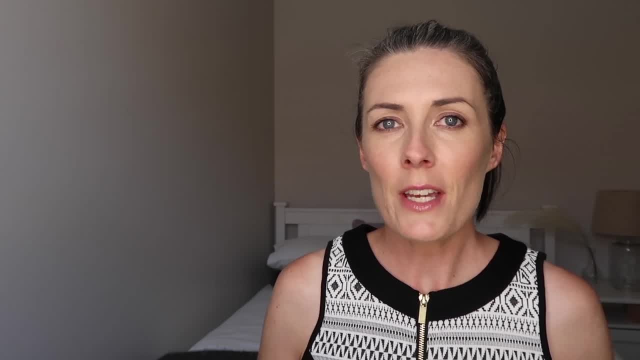 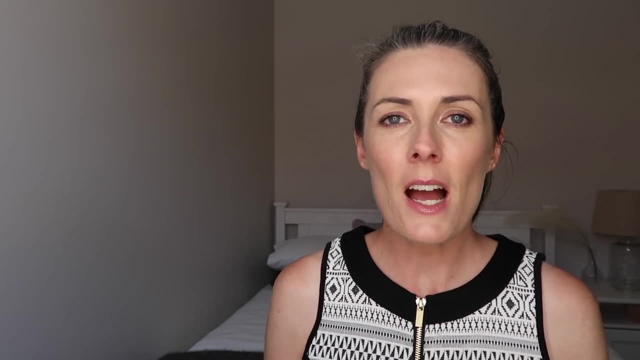 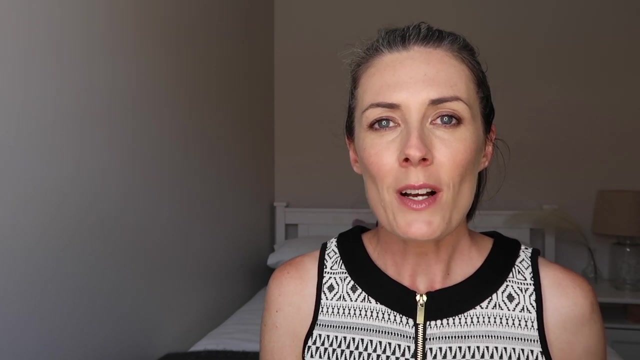 So within seven days I had created, written, illustrated and published a children's picture book on Amazon and it was available for sale And I had so much fun doing it. It was such a really great and fun creative process. So if you are someone who is creative as well- 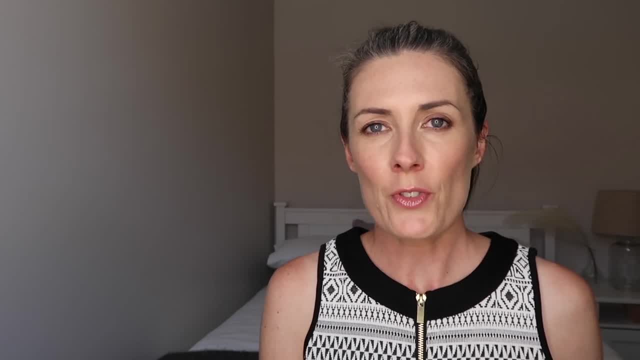 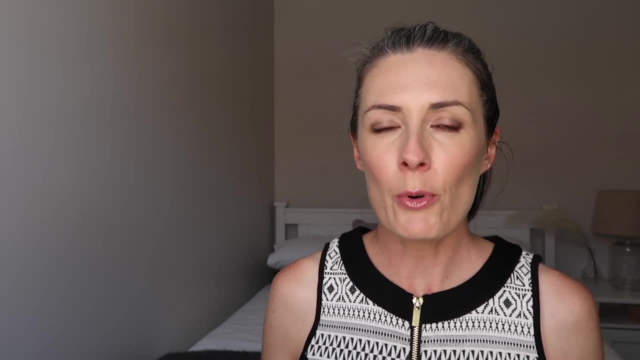 and really enjoys creating things a lot more involved than just notebooks and journals. you'll have so much fun doing something like this, And children's books can be as simple or as complex as you like. There aren't really any rules when it comes to making children's books. 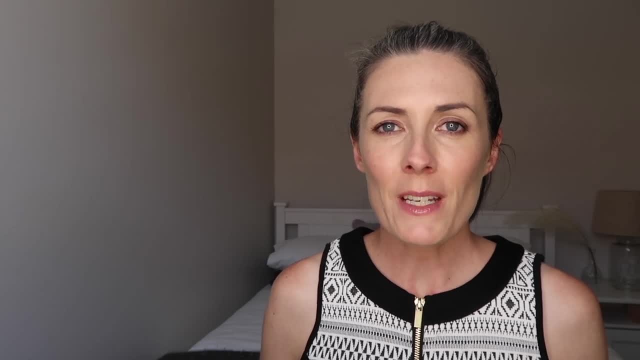 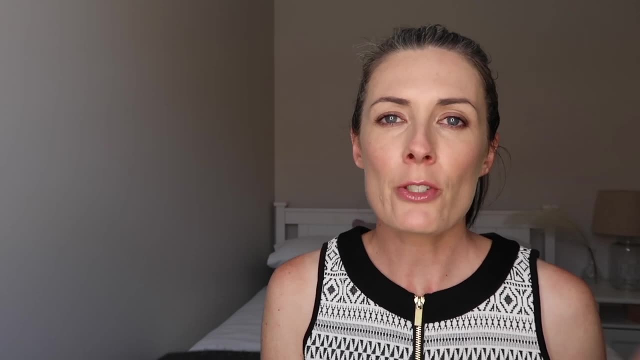 And there is also an unlimited amount of topics that you can write about. You might be thinking, well, I don't know what to write a children's story about, But when you sit and think about it or maybe do some research, there is so many things. 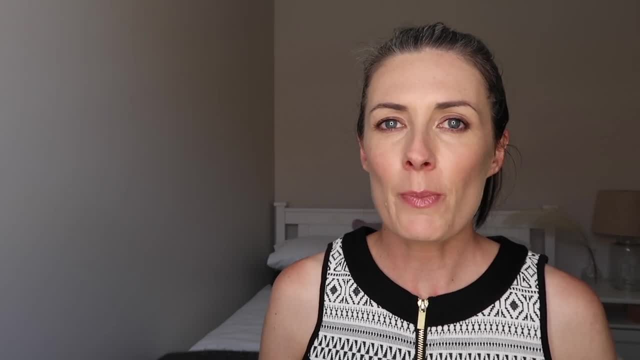 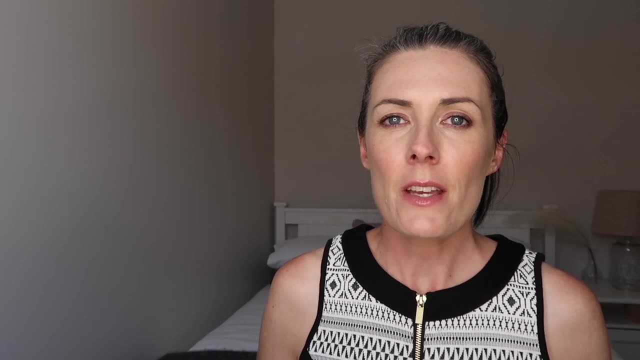 that you can create stories around for children. I know that I see a lot of parents out there searching for books that have stories that teach about morals and life lessons and basically trying to teach children how to grow up to be really good people. So you can write stories that teach. 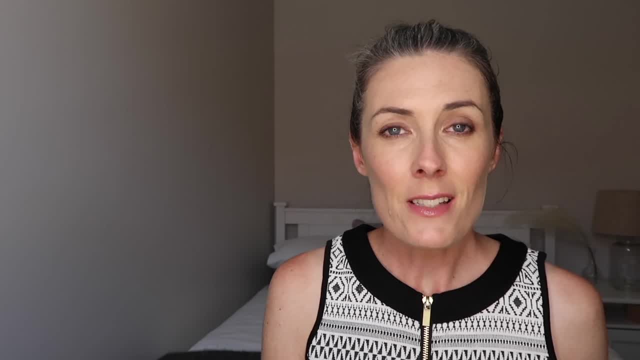 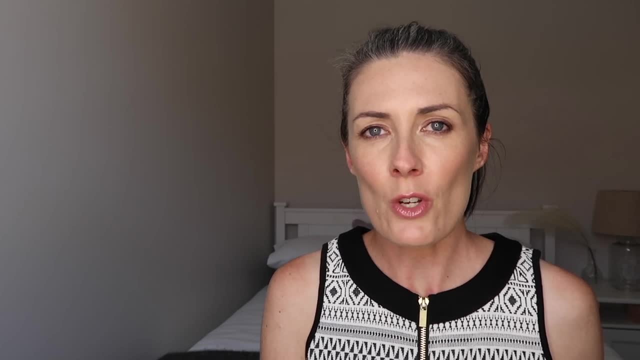 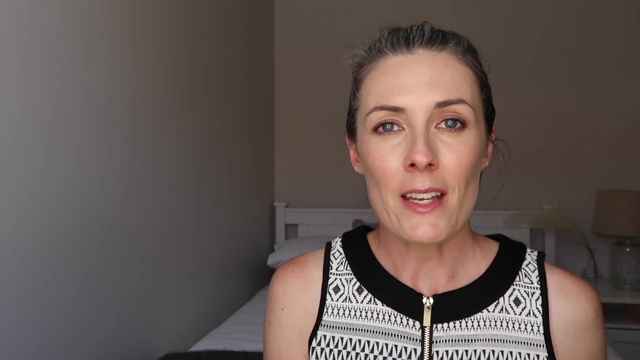 those sort of really important lessons within a story, But I don't know what to write about. But I also know that I read an article or I saw some information about a survey where kids were actually asked what they like most about books And the majority of them said: 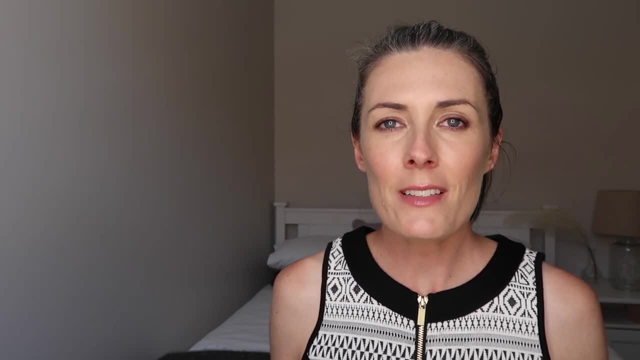 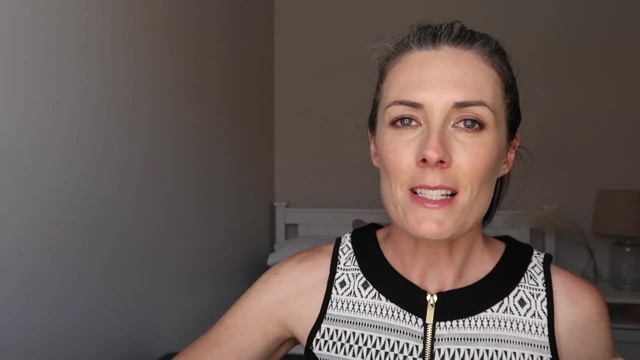 they just want a book that makes them laugh. So you can actually write stories that are about literally nothing, And as long as they're funny, kids will love them. I know that one of my little girl's favorite books is this one here: The Wonky Donkey. 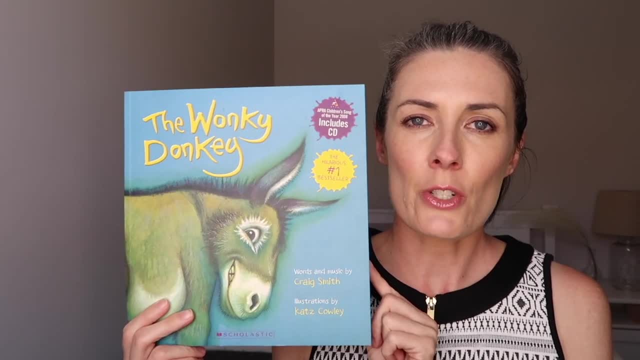 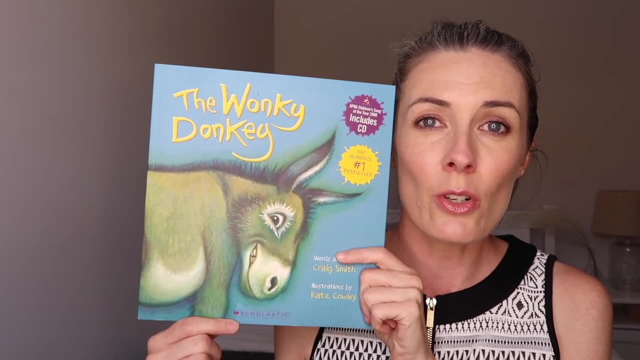 I'm not sure if this is available internationally, but it's very popular here in Australia And it's basically a story about a donkey with three legs loves coffee. he's really tall and he loves to listen to country music. If you're not a parent and you've never read this book, 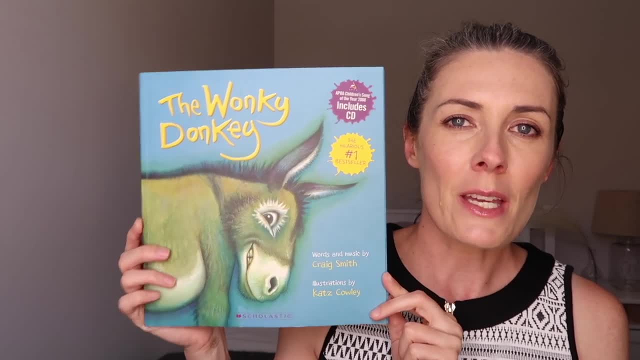 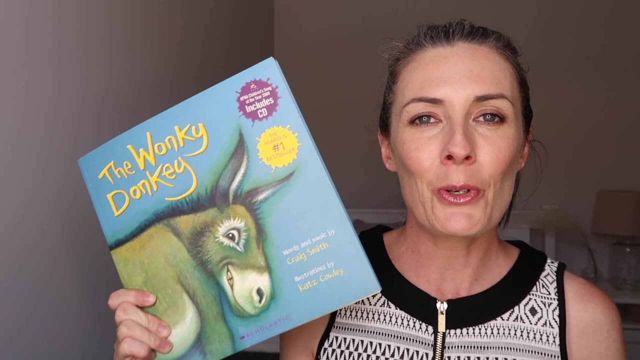 you'll have no clue what I'm talking about And you'll probably think I'm a bit crazy, but this book is about nothing and kids love it. And if writing just a funny kid's book about nothing is what interests you, then maybe try to find this one. 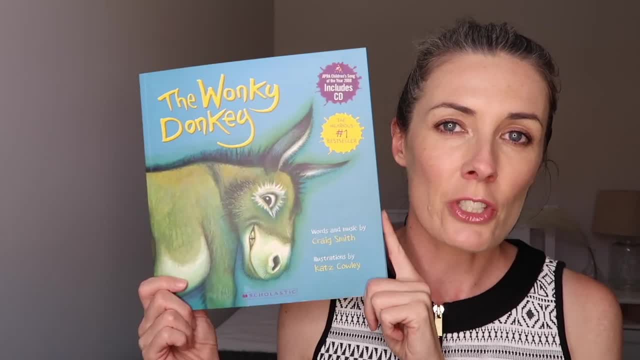 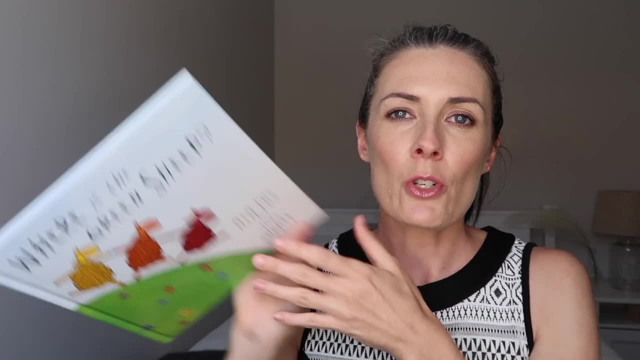 and just have a read of it. You'll be astonished at how simple it is. And with kids. just simple is better with kids. Now here's another quick one I'm going to show you Again. I'm not sure if this is only available in Australia. 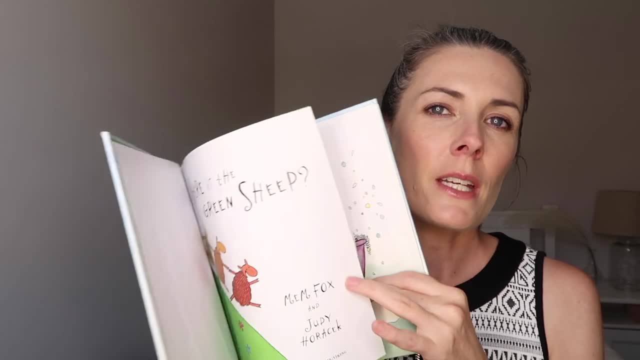 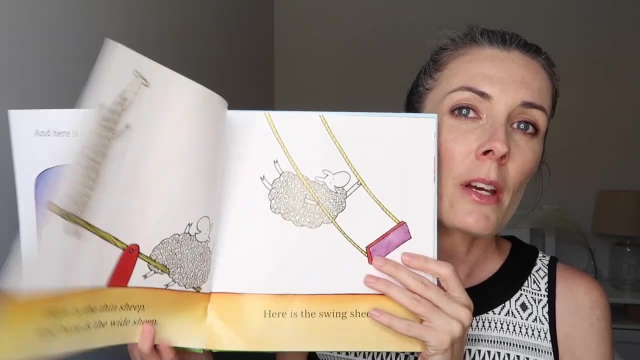 but this is called The Green Sheep And it is the most simply written and illustrated book. It's basically a book saying: here is the bath sheep, Here is the bed sheep, Here is the swing sheep, Where is the green sheep? And that's basically how the book goes until the end. 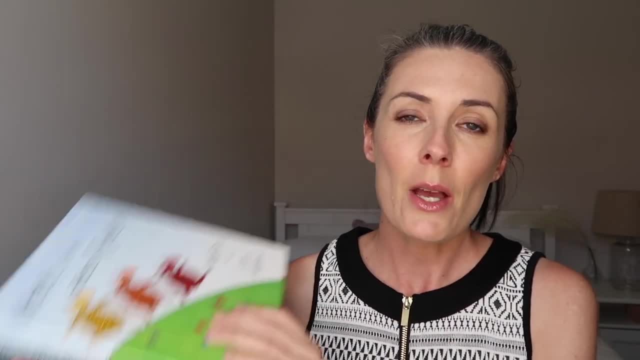 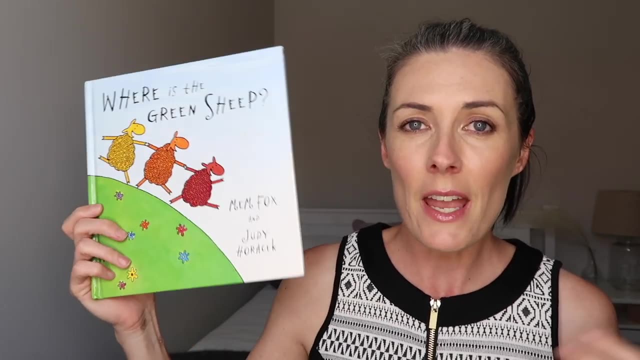 when do you find the green sheep? Well, you'll have to read it to find out, but simple, So simple, so simply illustrated. You would read this book and think what, Seriously, this is a bestseller. Anyone could write that. 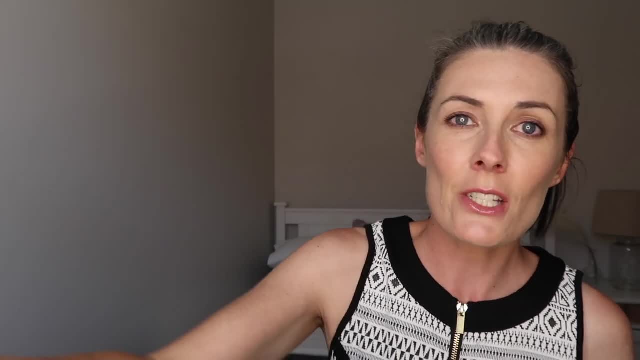 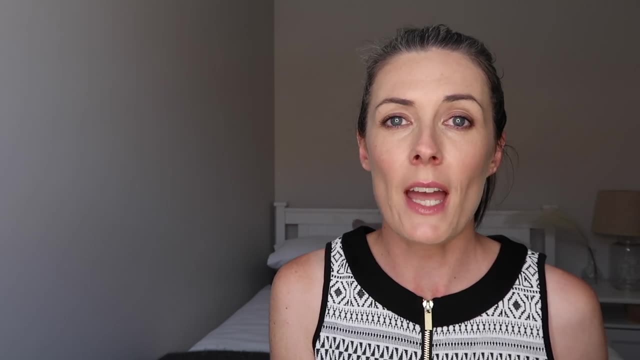 I could write that, Yes, you could. You just need to do it. So if you are interested in creating a children's picture book, then I highly suggest you do check out Nuria's course If you are interested. I have the link in the description below. 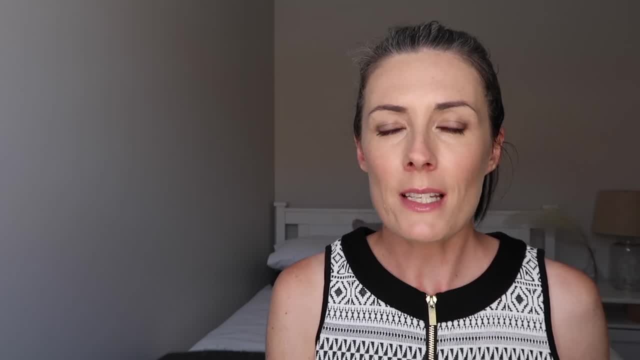 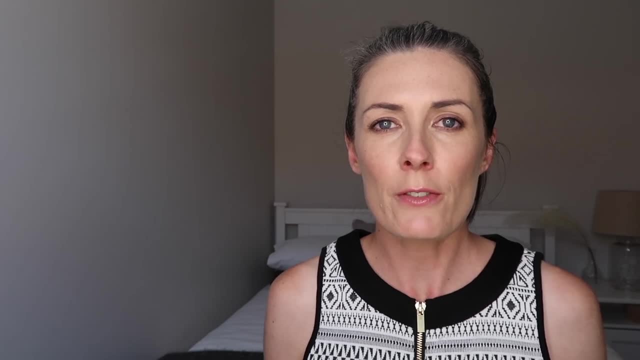 where you can go to her website and see all the information about what is included in the course and the pricing information and all that sort of stuff. It might seem daunting, And I think especially with the illustrating of a children's book when you think about creating one. 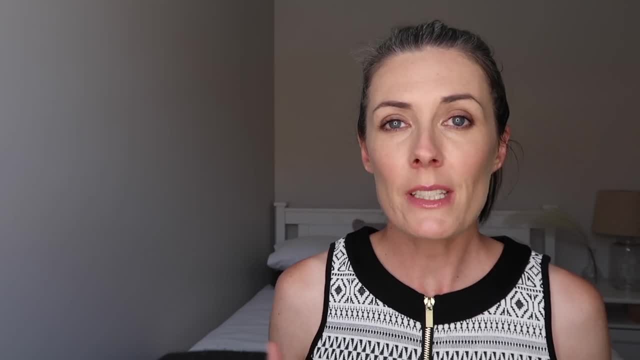 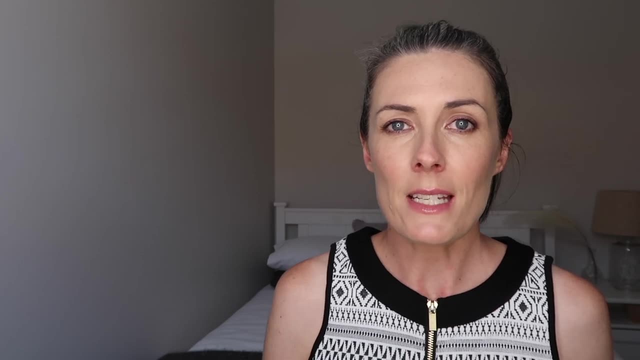 you probably think I just can't do that. I cannot illustrate a book, especially if you have never done anything like that before. But speaking from experience now, it really is quite simple and easy And, as I say, you can make your illustrations.